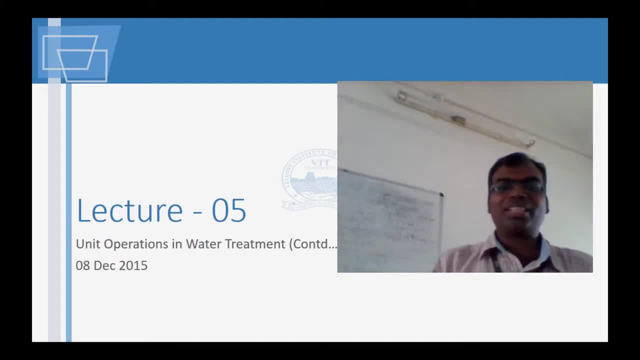 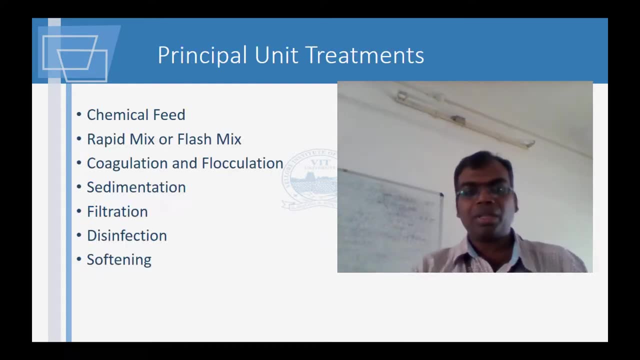 Good morning friends. We are just going to go very briefly into the unit operations which we already have done. So basically, this is what we saw. We saw there is a chemical feed. Chemicals are added for coagulation or flocculation and disinfection, Sometimes also to improve the feed quality. So these are the things which we usually use the chemical feed for. We have a rapid mix. We have also that is called flash. 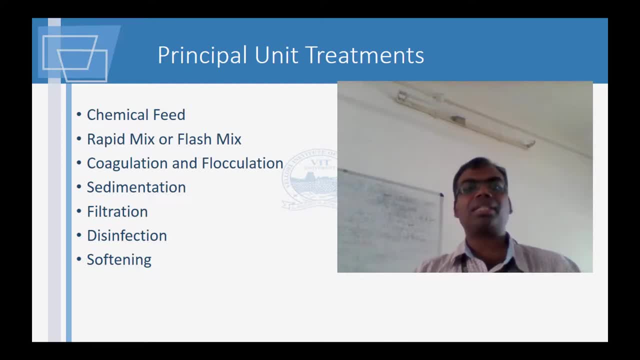 That is also. this is coagulation and flocculation. Coagulation: you add some coagulating agents which make the small particles to come together. You may add flocculant so that it forms flocs which you can remove from the water. Then there is sedimentation: Big particles are allowed to sediment. And filtration where you pass it through a filtered media. Filter media will hold off all the substances which cause coagulation. 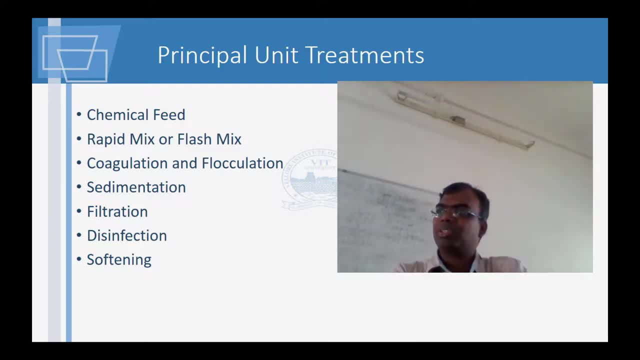 Also turbidity and particulate materials and also inorganic material. So please remember this. activated carbon is not a disinfectant, It is an adsorpting agent. Absorption is a surface phenomena. On the surface of it it can take many of the chemicals And many of the inorganic chemicals get adsorbed on it. So taste and flavor get improved because inorganic materials get adsorbed on the surface of activated carbon. 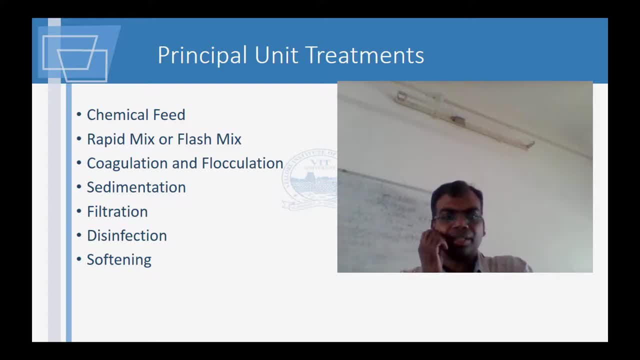 So then we have this filtration and disinfection. Yes, you know what disinfection is The most primitive, or what I will say is one of the oldest disinfection technique is chlorination at home Boiling. In fact, somebody had sent a message on WhatsApp also. 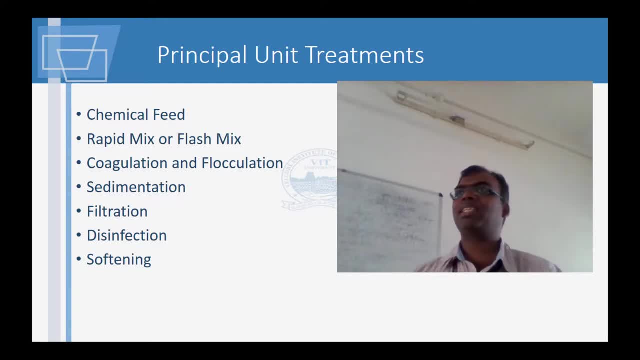 Take water in the pressure cooker- 15 whistles. Even the worst of the pathogen is going to get killed. That is also called as auto cleaning. That was the message. So I am just putting what they told me And I am sure that you will understand that it is one of the most effective methods of treatment. 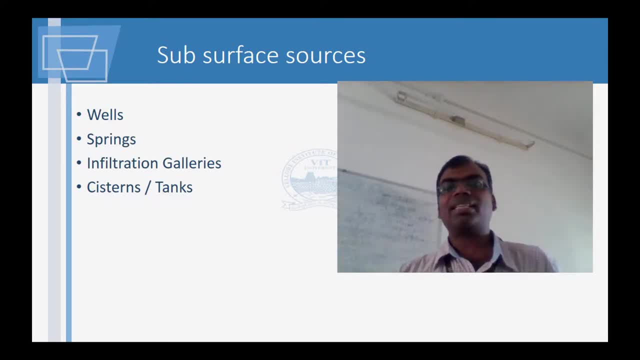 So we were talking about subsurface sources. Infiltration galleries are nothing, but sometimes they are Like huge rooms itself, with holes into which water can collect. It will form a channel and then they collect the water. Cisterns and tanks are used for storing water, or rain water specifically, So in India we usually call them as tanks. If you are using some of the foreign author books, they are using the word cistern. 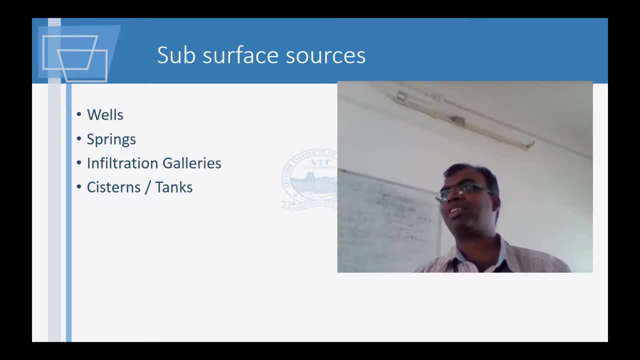 So in every village we actually have a temple. normally There is a huge tank And almost In most of the cases, if we are not interfering with nature, you will find that the tank is going to be filled. So basically what is happening nowadays, all of us want to have the comfort of having the water from our own house. 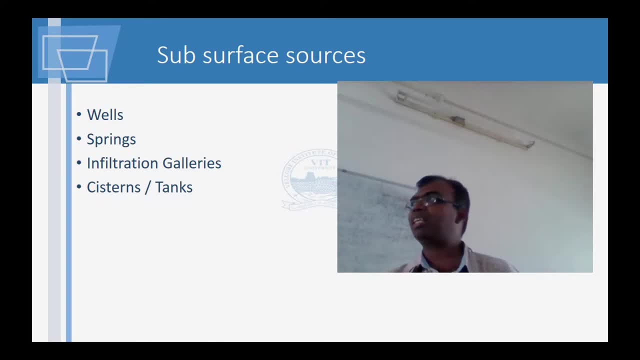 So we dig a deep well and if you remember in hydrology you would have studied that around the well there is a local depression of the water. So if this keeps on happening, the ground water itself keeps reducing And all these tanks are getting empty. 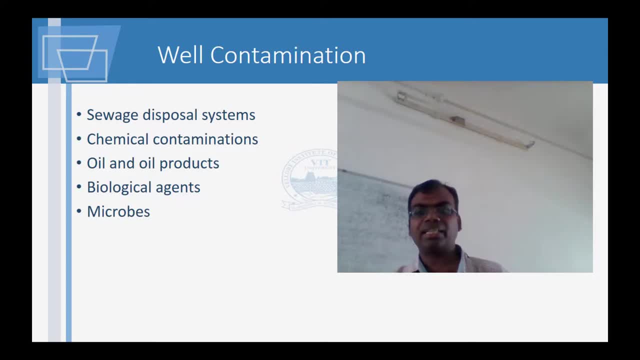 So anyway, so these are the things where this is how the wells normally get contaminated. This is the way the wells normally get contaminated. So what do we mean by the sewage disposal system, For instance, if you are having a septic tank very close to your bore? well, 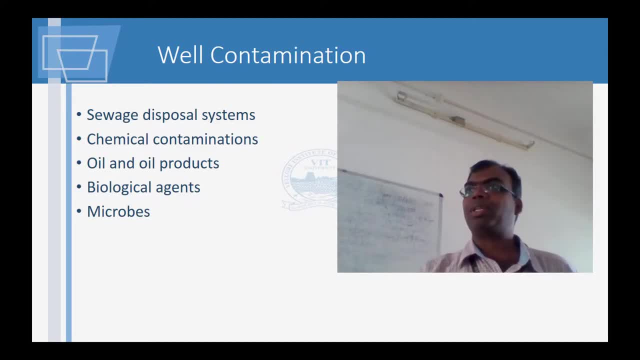 You are definitely going to pollute your bore well. So this is just a simple example. But there are other sewage disposal methods Also which, when the thing is subsurface, When the thing is a subsurface system, you are going to have the water getting contaminated. 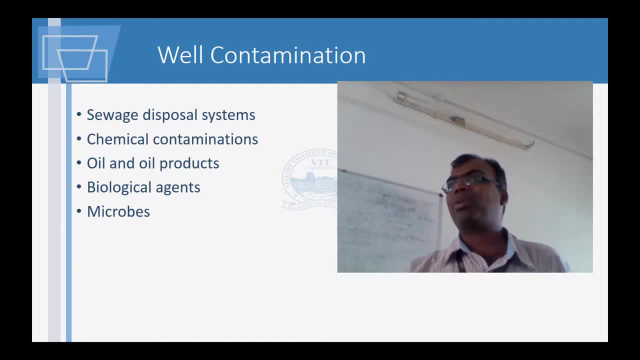 Contaminated by pathogens, like whatever is in the sewage, Especially coliforms, what we talked about, coliforms, And they cause diarrhea and all those diseases. And how do we do these wells? How do we dig wells? You know that right. 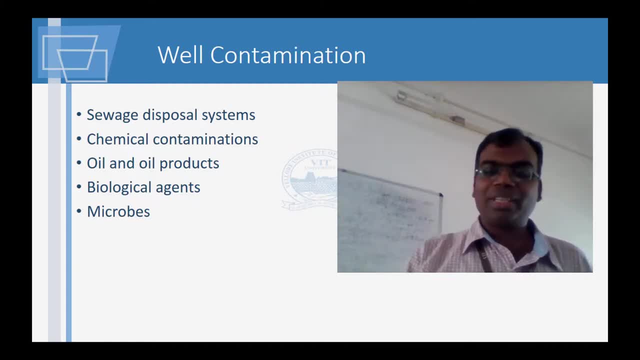 So traditional methods are there, Bore wells are there now And then. we also have chemical contaminants, For example, In In any of these near these pharmaceutical companies. Whatever they put in, Including, like this, pesticides, They all get washed down into the water. 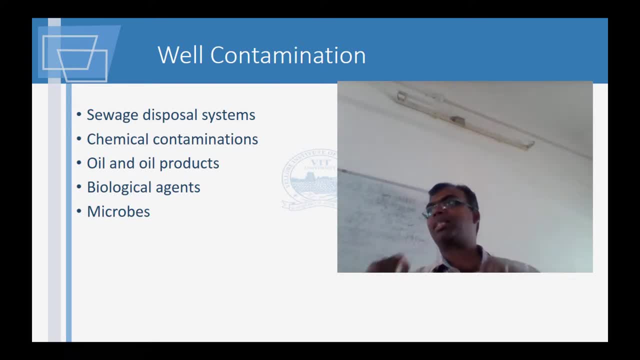 Pesticides don't break down easily. Their chemical structure is such that it is so strong It is still not break down easily. So, and also, they are water soluble. In fact, that is what they want. They want it in a way that all these insects will get the pesticide. 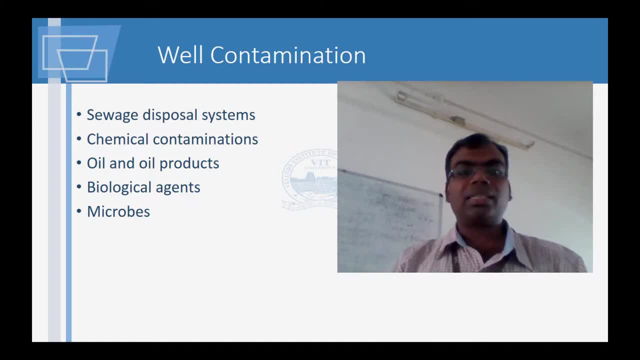 In the process we also start to get the pesticides, Oil and oil products. I don't know. I don't know if suppose you are familiar, But in the Endor side There is a huge refinery, Madras refineries MRL. 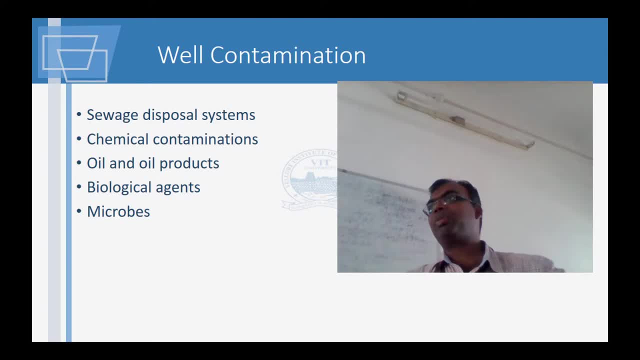 Now I think they call it Chennai refineries, Whatever, But they have huge pipes conveying oil from the port to the refinery facility. Some of these pipes have got leaks, So all these leaks have spoiled the ground water in that entire area. Purukpet, I think, is the name of the place. 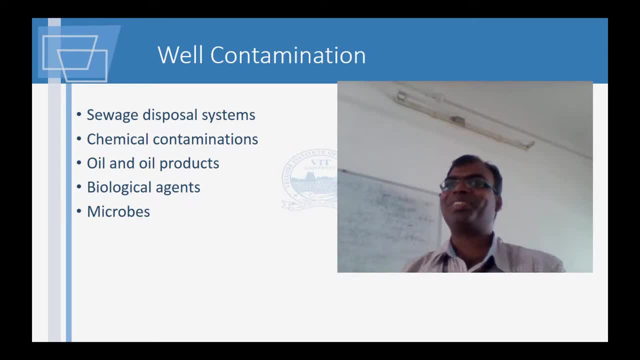 So people are all complaining that they are having oil, Oil. Very sad. no, We are saying no oil. These fellows are complaining about oil Anyway. So can you think of the remediation? It is very difficult. So this is also gone into the ground water. 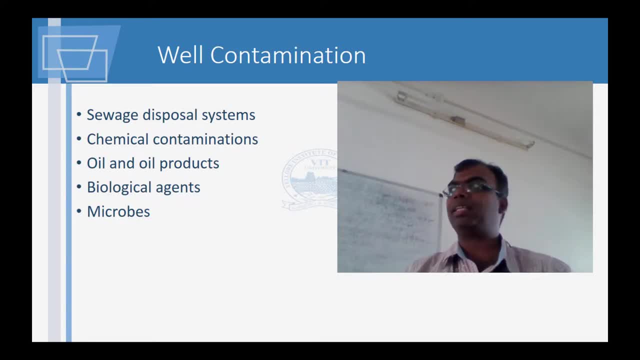 And biological agents. Biological agents are many, In fact. what I was reading, I was reading somewhere: Notice we are taking a bore well Which goes very deep into the ground. Well water is one of the purest forms of water. Why? 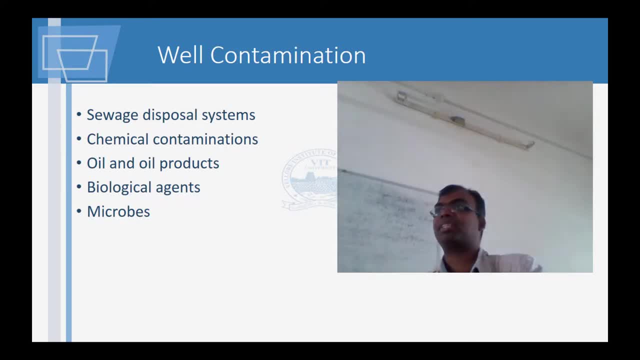 Because it is actually having a very huge sand filter. It goes through the sand filter before it reaches into the underground storages. Now, what we are doing? we are drilling a hole. Any bacteria and virus can just go in and contaminate the source. 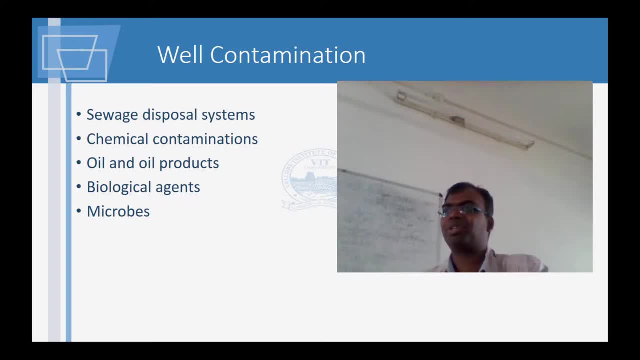 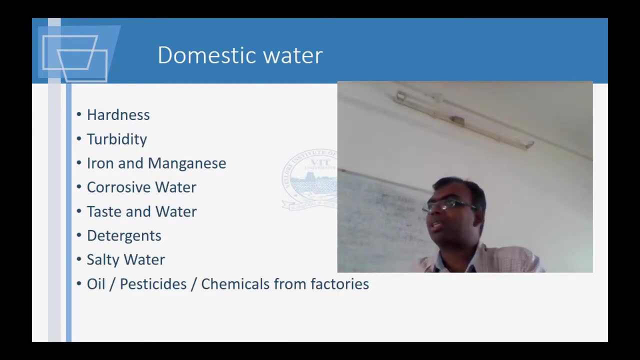 So this biological agents and microbes are a very big problem, personally, in my view. Next we are having the domestic water. The domestic water problems hardness. hardness doesn't let suds, it forms suds. Hardness also makes the water pass, scaling in pipes, Most of you know. if suppose pipes keep dripping, you will be able to see salt formation itself at that thing. 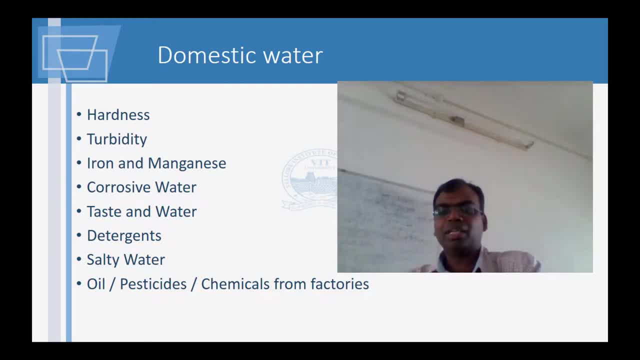 This tap won't close properly. So all these are some problems which we have And also we don't know. it is this calcium and bicarbonates, magnesium bicarbonates- that cause it, And the issue is you can also get things like kidney stones and stuff like that. So we cannot actually it is not acceptable. 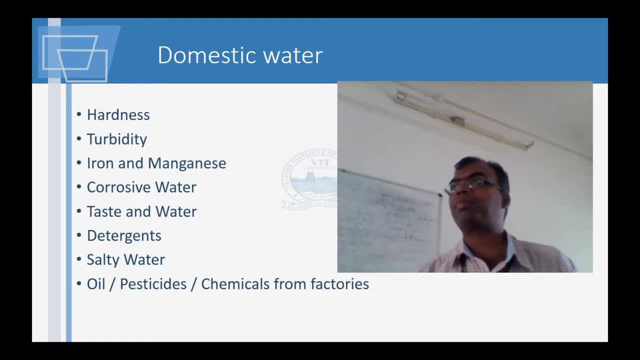 So we usually use something like probably zeolite processes at home. Ok, EDTA, all those things. This may be possible on a very large scale. You would have studied this in chemistry. So now on a home level, for iron and manganese also, we use this zeolite columns. Ok, So it will remove the iron and manganese. The problem is it will cause that alloys, stains and all these, And of course they are not also good for humans. human consumption in large quantities. 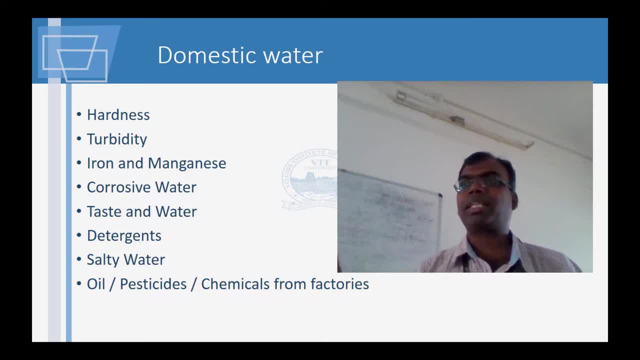 And turbidity filters, activated carbon that will take care of it, And also the other filters. If you look at your aquacard and all these units, you will have a pre-filter. So it is nothing but layers of some membrane which is there And you pass through the membrane, you will get a clear water. 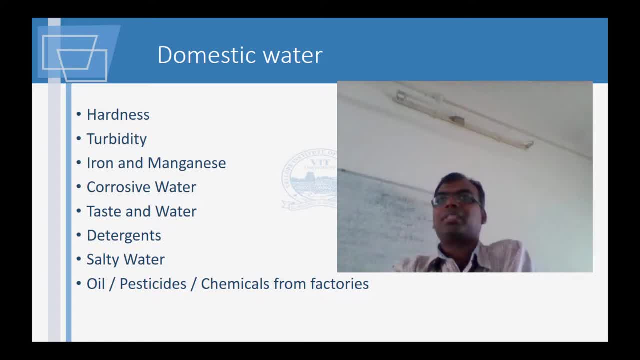 Then corrosive water. it corrodes the pipes. steel pipes will get corroded. So you may, you will have to add some basic substance to make it, to neutralize it. Ok, Ok, Ok, Ok, Ok. So taste, it is not taste and water. taste in water. Ok, Taste and odor also. It should have been taste and odor. I do not remember. I do not understand how I made it that way. 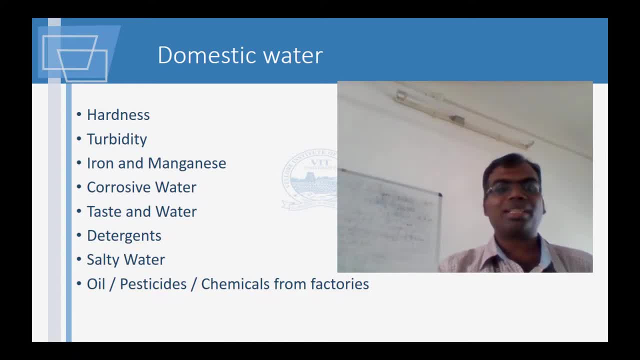 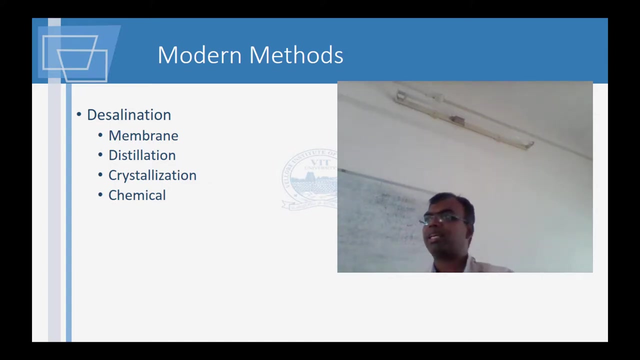 And detergents. you know what they are. what they are: Salty water And oils, pesticides and chemicals from factories, So places like Bhopal, and all including the groundwater. everywhere you are having problem, Ok, Ok Now. so these are the techniques of desalination. Ok, You are having ion exchange, You are having electrodialysis, You are having reverse osmosis And you have ultrafiltration. Ok, 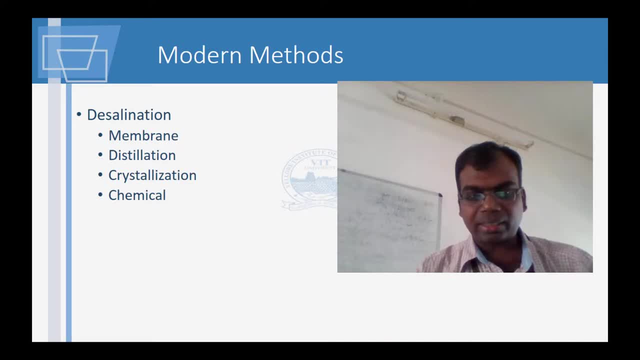 So I am going to add this also: Membrane techniques of water treatment. Ok, These are all water treatment techniques for domestic water, drinking water. So I want you to just go in for this: What are the membranes which are available commercially for for our water treatment? Ok, 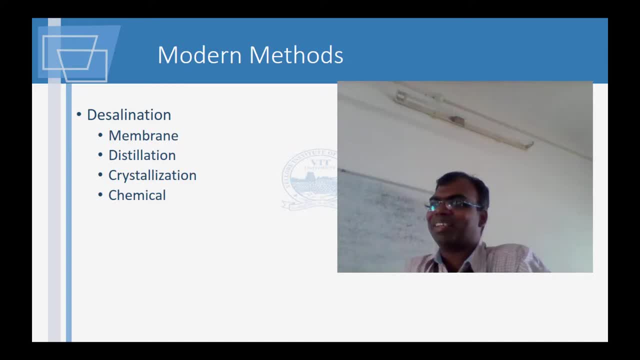 So I am telling it again: It is not in your notes. Membrane techniques: you should be familiar. It is very simple. Since it is also, it is all in first-take industry, right? You do not have that. 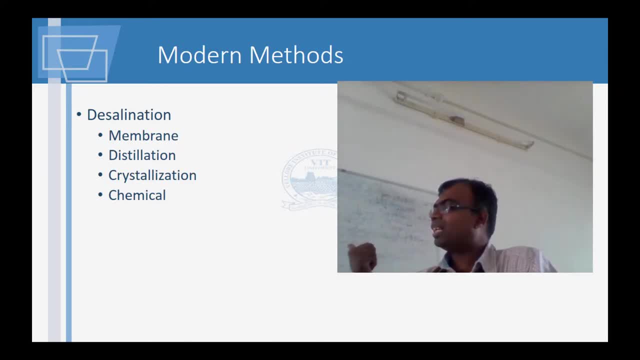 Ok, Ok, Ok, In all these cases, in any case, you look up your books, study it. Ok, Because it is, it is very, very, very fun. Ion exchange: reverse osmosis: Ok, Osmosis where? 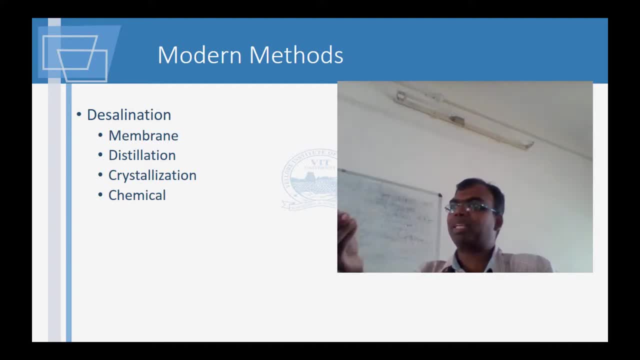 Yeah, That is because of the pressure gradient across a membrane. Ok, This is what osmosis, from region of higher concentration to region of lower concentration- goes From. here you are going to do the vice versa, Ok. And then they have ultrafiltration. It is nothing but passing it through very fine, in order of few microns. they have course, Only water can go through. In fact, bacteria gets filtered out of that, but some virus can go through it. And then you have electro-dialysis. Dialysis is also a membrane, like osmosis, So it just go through that. 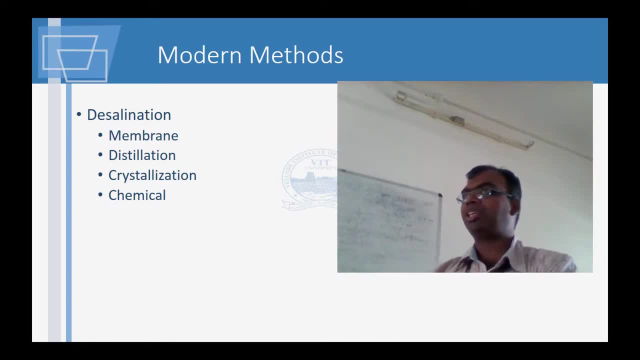 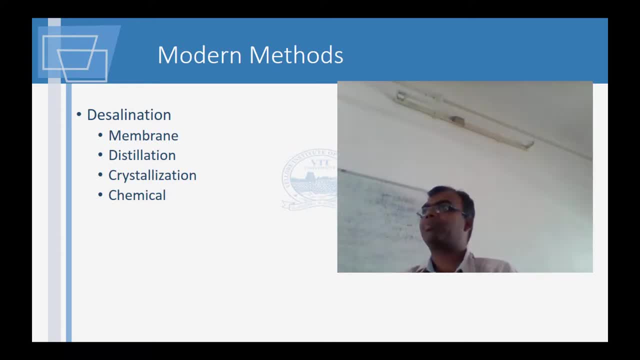 Ok, Ok, Ok, Ok, Ok, Ok, Ok. places where they have huge domes, ok for distilling water, and then they based on the solar energy. the water goes up, it gets condensed on the dome and it slides to the sides. 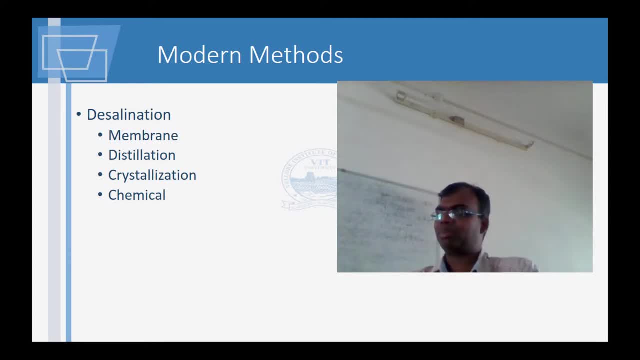 So salt gets formed in the chamber and water is taken out. So sometimes they freeze the water and then they are able to. they do it at a eutectic point, ok, So at that time they are able to separate the salt and water and then they are getting. 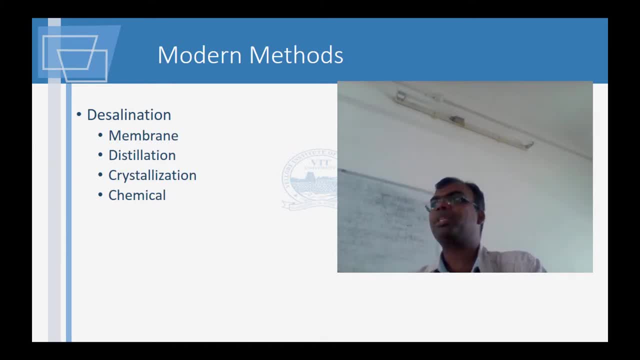 some fresh water. Same thing, some chemicals can be added to depends on the feed. you add some chemicals and then you are going to get the fresh water. I am not going to ask you about this chemicals, chemical treatment method, but I would like you to know this. membranes- look at the distillation methods, ok, and crystallization. 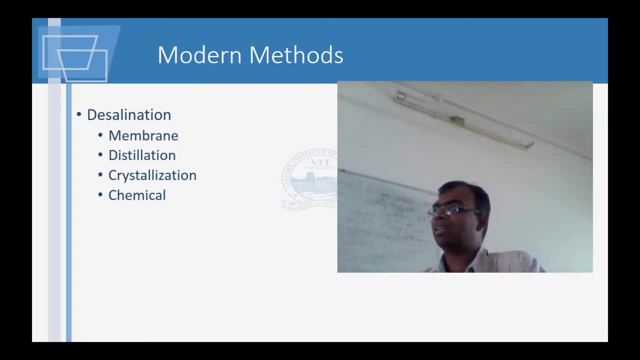 Crystallization technique is nothing, but you form crystals. You form crystals and you get the material which is inside and the materials that cause the hardness- water of the salt which is dissolved in water, and they remove it. Next is pretreatment of water. 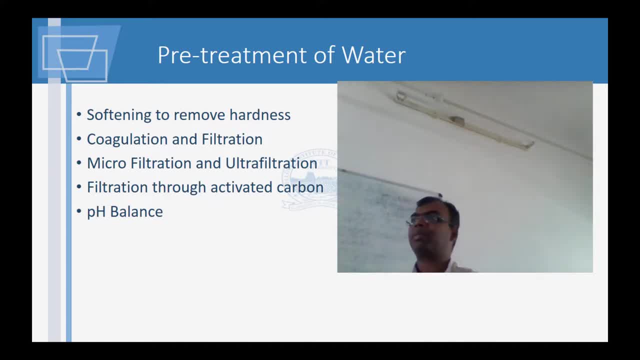 So, basically, if hard water is there, the performance of the treatment plant is very badly affected. So we try to remove the hardness. ok, it might be EDTA method or any method, depending on the degree of hardness and depending on the efficiency they want the hardness to be. 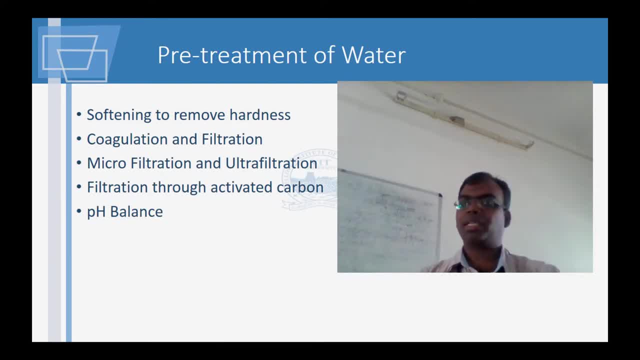 So this is the method. So this is the method. So this is the method. So this is the penurst, Simon. Then you got coagulation, Then you filter off, you run the filtration- micro filtration, ultra filtration are done to remove the particles that cause turbidity. 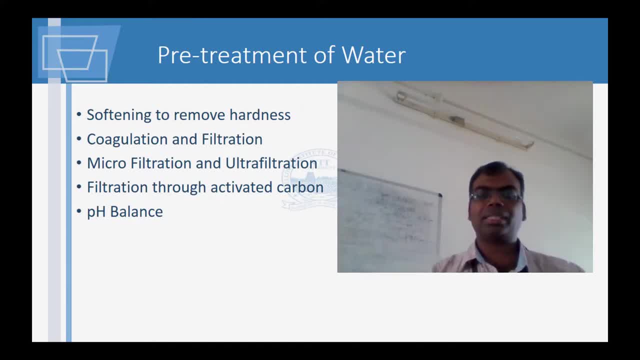 Ok, Any of the floating particles can be removed by using these techniques. And then, please remember, activated carbons only to remove chemicals. Ok, chemicals, sorry. Can you say that, Sir? I don't know whether I can call that as micro filtration. I don't know, because many times 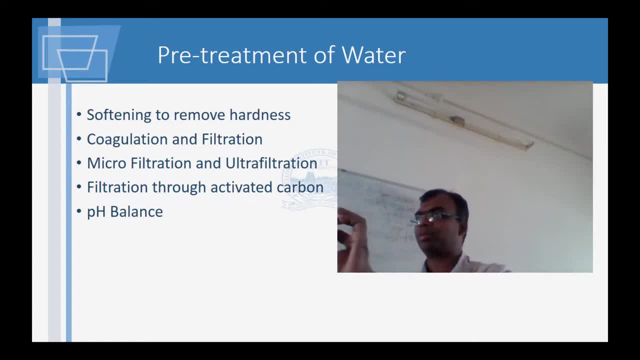 activated carbon is a small size, particle only, But micro filtration, normally, by what I have read, because I am not an expert, frankly, in water treatment. Actually, what happens in activated carbon is whenever you are having something like micro impurities, A chemical agent, See. 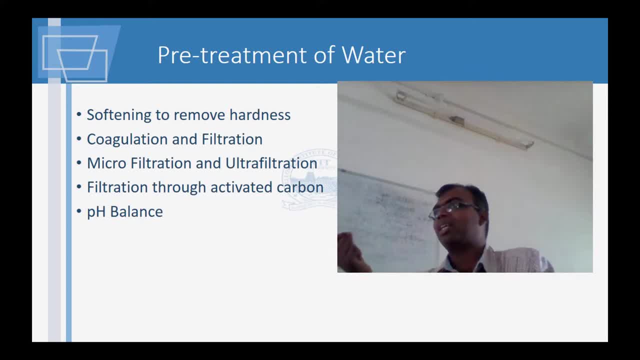 So the concentration is very, very less, which you can't normally remove with the ordinary thing. So in that case, yes, I bow your argument that it is micro filtration will hold water. I agree, I agree, But I can't put it under the same category because the principle of 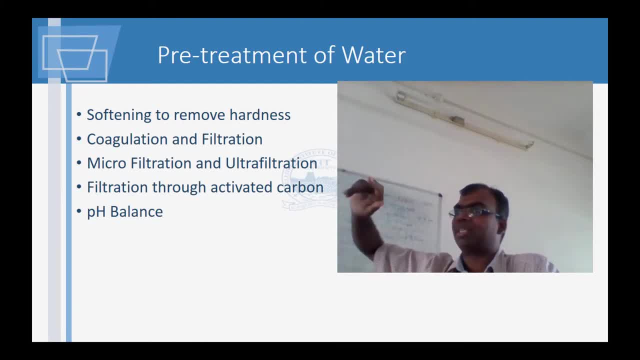 activated carbon is. it is a surface phenomenon, The other one is a barrier. Sizes above a particular size is not allowed. Ok, It is not allowed to go through, Ok. So if you look at your seam analysis, it is a mechanical process by which it is held out. 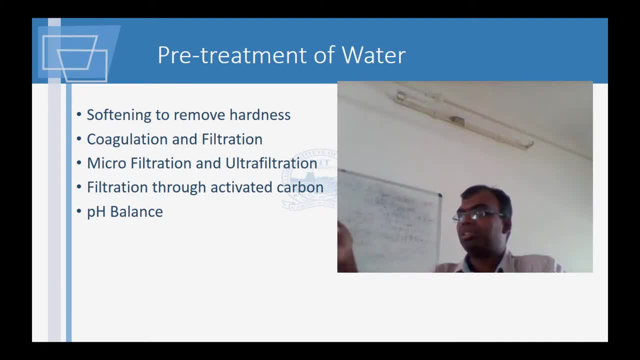 But here it is a chemical phenomenon. Absorption is used to hold it, So how it is going to matter- whether it is ultra or micro, I don't care, But what I want you to know is this is a surface phenomenon that is more of a mechanical phenomenon. Sometimes you suck the water with a lot of. 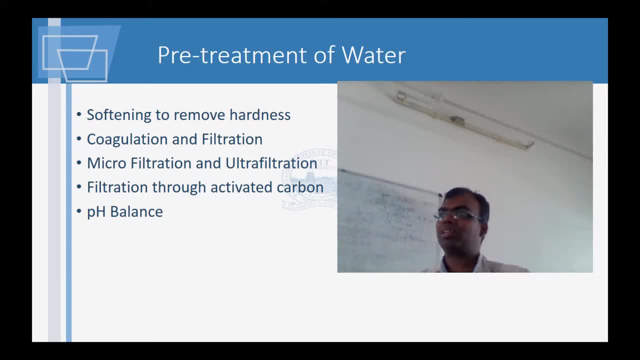 vacuum pressure through the pores and then take it, Or you create a high pressure on the outside so that the water tries to go in through the. it is squeezed the water into the pores. Please remember that video which we had yesterday with that water property that was saying no. 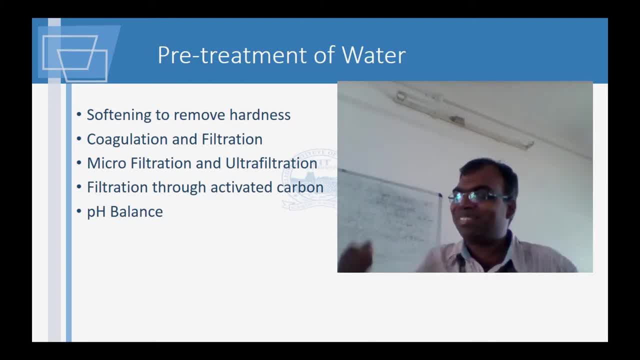 this is very painful. She made to squeeze it, squeeze through. Next we are having pH balance. ok Again. many of the processes, for instance- I will just revisit again- coagulation and all these things- You will find that there is something called zeta potential. I have not talked about zeta potential, But I hope I want you to go and 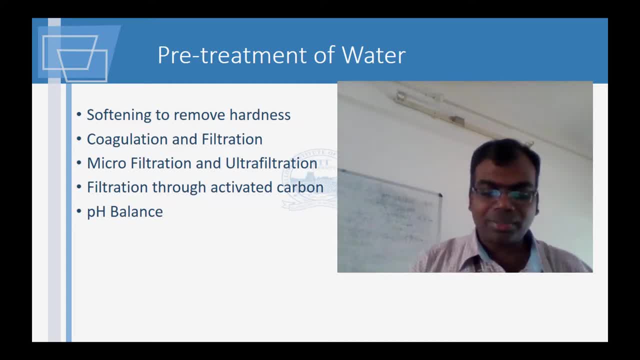 look into your book for the word Zeta potential. ok, In fact, you might even take it as an important thing, because I am making a note of this right in front of you guys. I don't know where I am going to ask, but I am bound to ask this sometime. I mean to. I want you to do this. zeta potential- What? 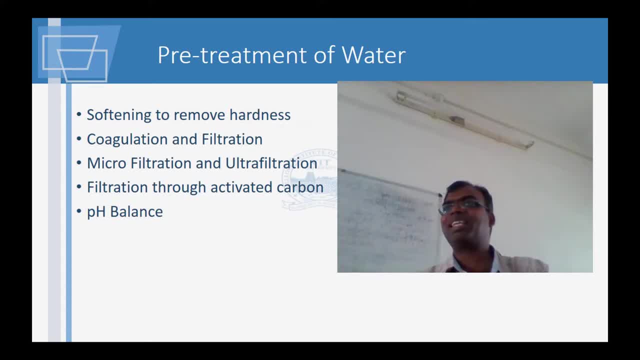 is this zeta potential? Basically, we are telling that we have to form flocs and all these are small particles which have to get acclumarated. Nice word- again, I am using words which I didn't know. I knew. Ok, good Now. acclumaration is to enhance the process. you can just form. 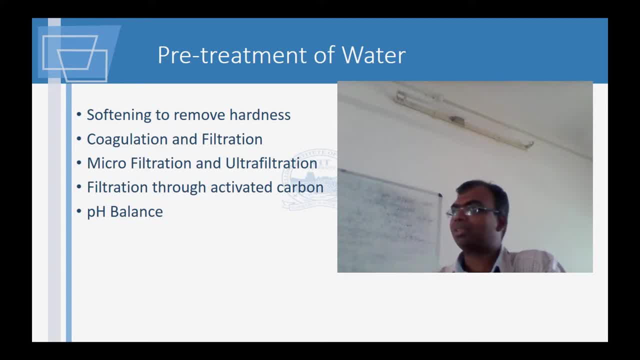 you can have a electric current fast through the liquor. Liquor means the fluid which is there in the chamber. We have a zeta potential, ok, In coagulation. you will be able to see this. Yes, yes, see. this all enhances the efficiency. This all enhances the efficiency of the process. 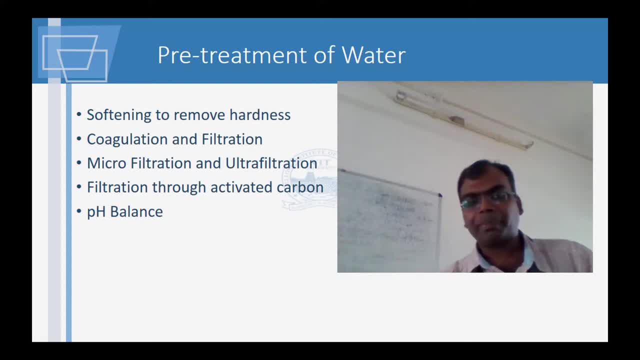 It makes it go quickly, basically ok. So that is why we can use that. But just remember in one of the videos they had that coagulation agents. they ran water very, with very high speed. Did you notice how the settling took place? it was so rapid. So nowadays the materials: 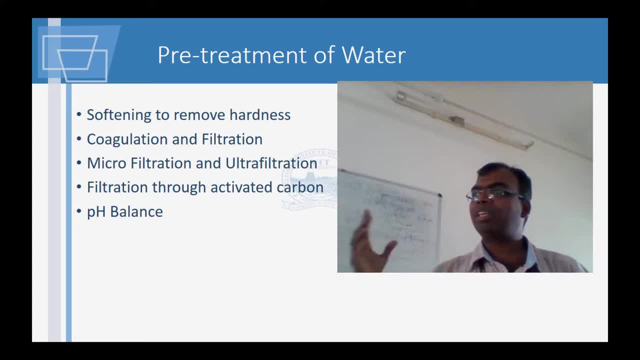 which we have, some of the, sometimes polymers are being used. So these are the materials which we have, very good and very effective materials nowadays. But to get it to work, to get them to work, pH should be there at a particular level. If suppose there is a lot of turbidity. 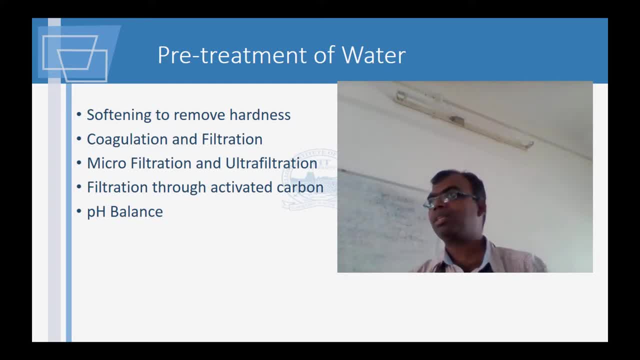 ok, the larger size particles are there. they may disturb the process. So that is why we may have to, we will have to choose mix and match to get a right fit At this course. in this course, we have to know that such a thing exists, How it is going to or what is going. 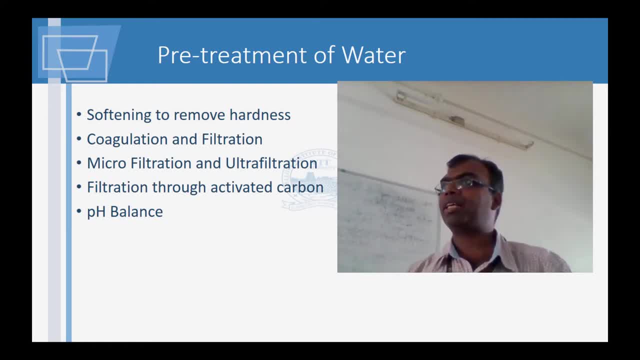 to be done might be important if you are going to take a public health engineering or a environmental engineering course as your masters. So there you will be, having to know what and what should be put together, what and what should not be mixed together, or you can yourself design. 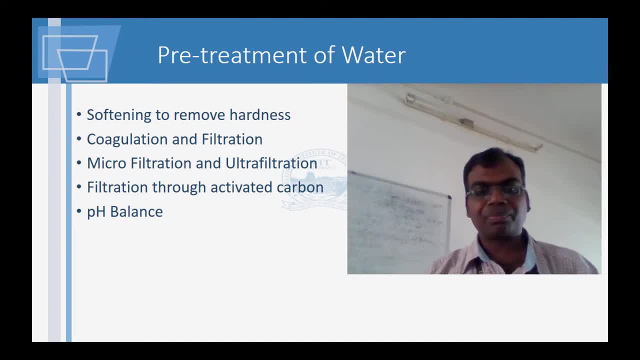 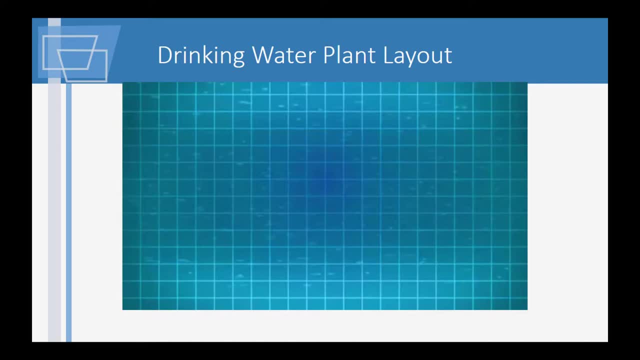 a new system which you can, which will work. I am just going to go through a drinking water plant video again, So I hope you enjoy it. Welcome to our tour of Winnipeg's drinking water supply and treatment system. We use leading edge technology to treat the water as it passes through many stages, including coagulation. 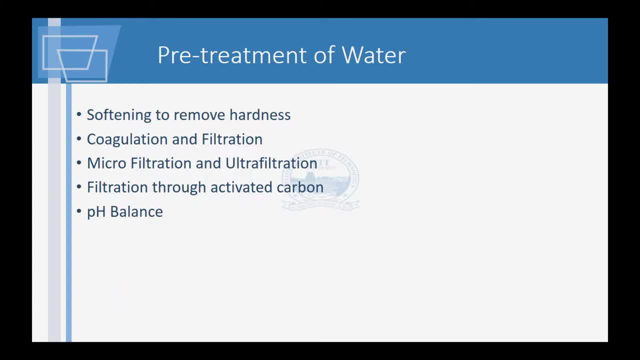 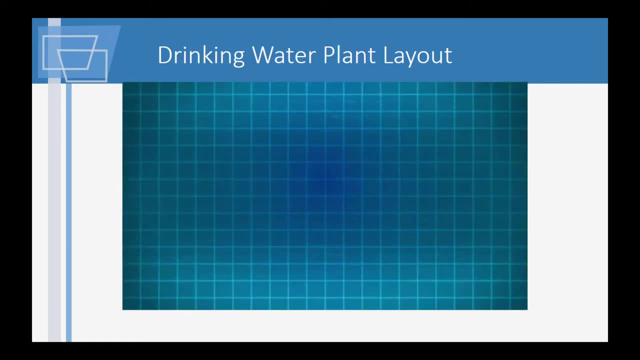 I will just play this again because I am sorry the volume was turned down low. Welcome to our tour of Winnipeg's drinking water supply and treatment system. We use leading edge technology to treat the water as it passes through many stages, including coagulation. 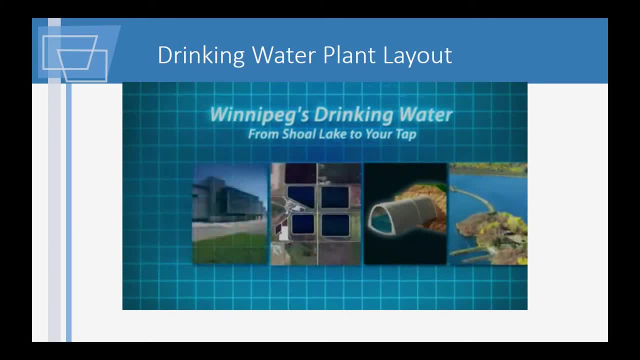 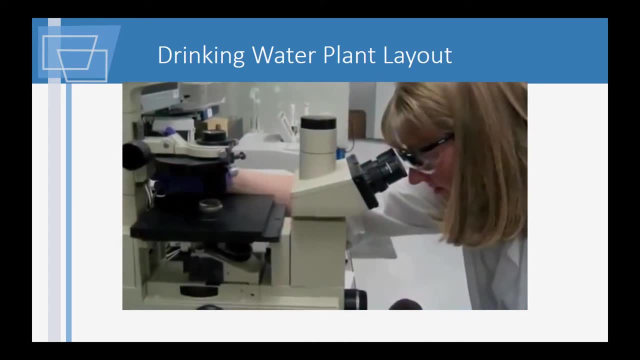 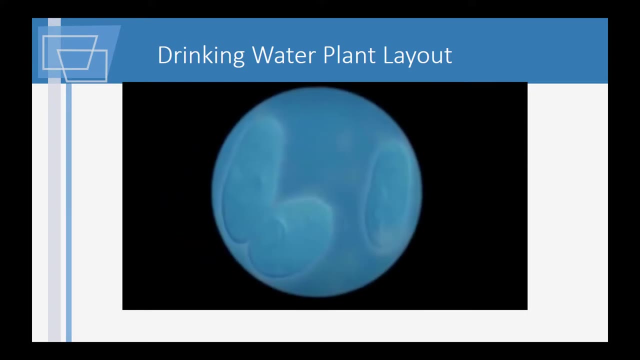 flocculation, dissolved air, flotation, filtration and three types of disinfection. Our system protects public health by virtually eliminating the risk of waterborne disease and reducing the level of harmful disinfection byproducts. It also improves the taste, odor and appearance of our tap water. 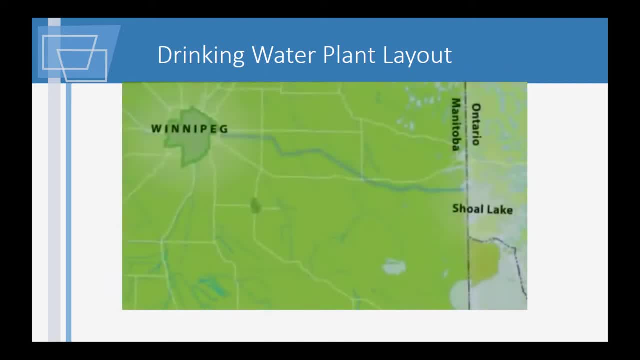 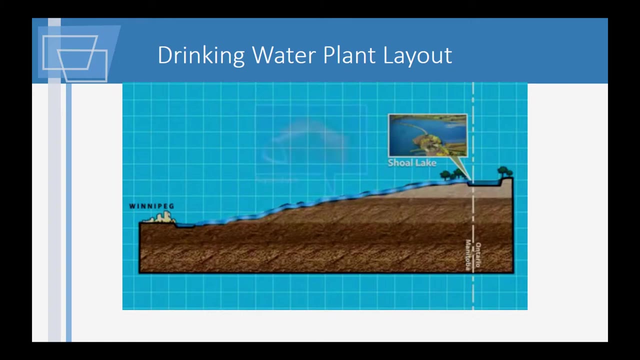 Shoal Lake has been our source of water since 1919. It is located one mile south of the Winnipeg River. It is located 136 kilometers from Winnipeg at the Manitoba-Ontario border and is approximately 92 meters higher than Winnipeg. Water flows downhill from Shoal Lake through an aqueduct into four large reservoirs. next, 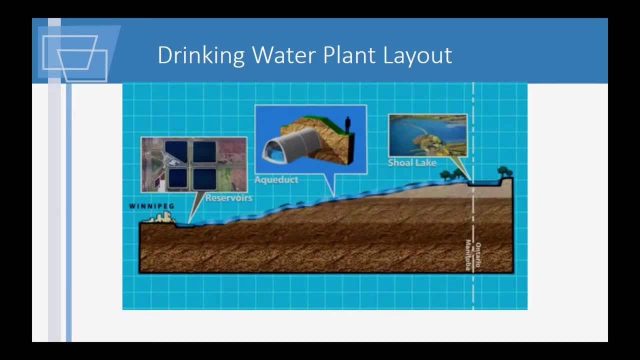 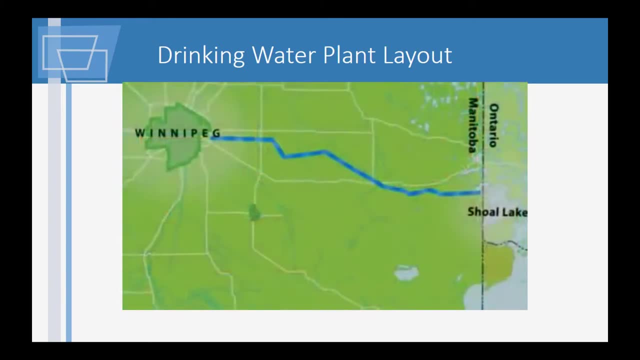 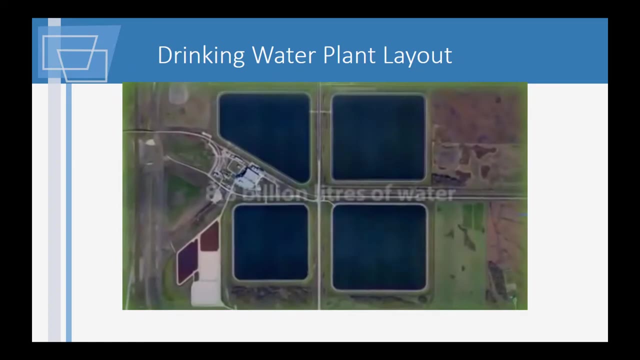 to the treatment plant. The aqueduct is a large concrete pipe that carries up to 386 million liters of water per day to the reservoirs. The reservoirs hold up to 8.8 billion liters of water, which on average, is enough to supply. 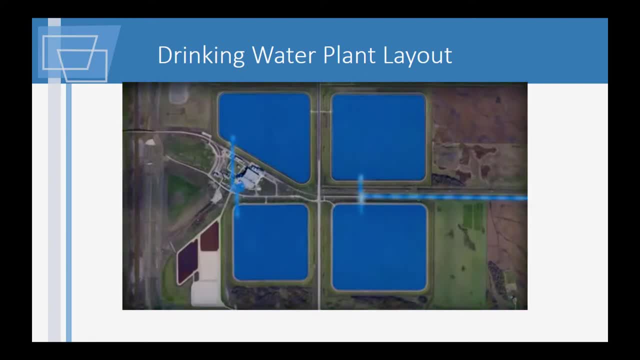 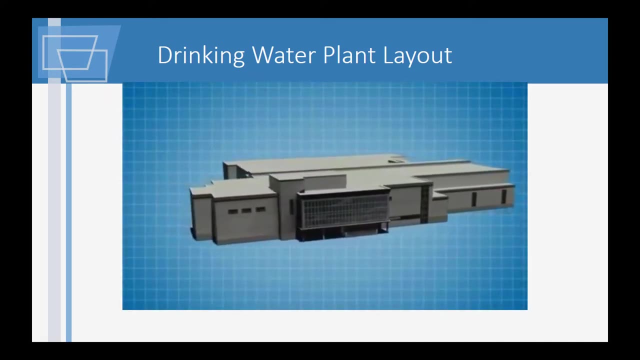 Winnipeg for about 30 days. Water flows from the reservoirs through two large pipes into powerful pumps that move the water into the plant for treatment. This $300 million state-of-the-art facility features a highly automated system that monitors and controls a wide variety of instruments, mechanical equipment and electrical equipment. 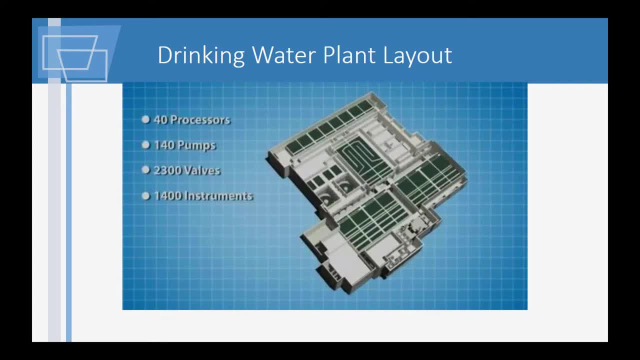 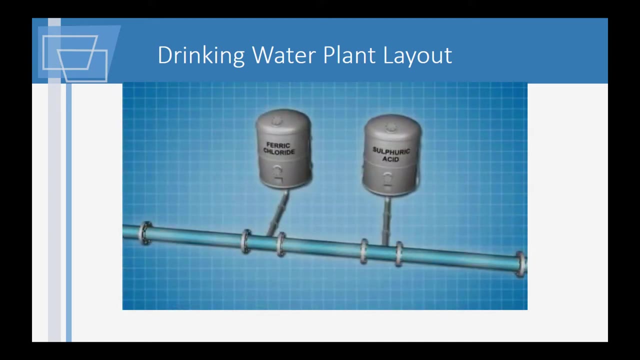 including 40 processes, 140 pumps, 2300 valves and 1400 instruments. It can treat up to 400 million liters of water per day. In this first step, we add sulfuric acid and ferric chloride as the water flows into the. 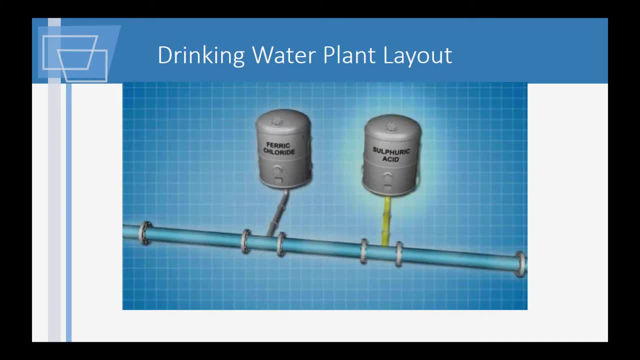 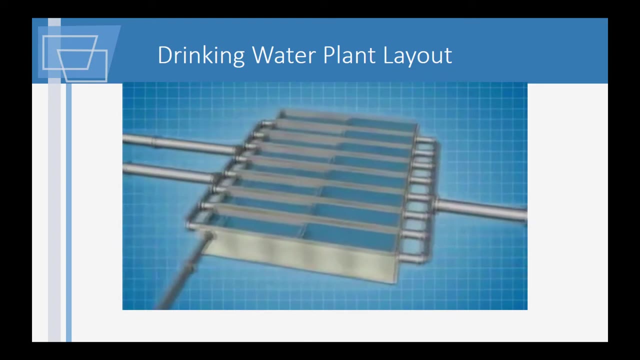 plant. Sulfuric acid lowers the pH of the water and makes this stage of treatment more efficient. Ferric chloride, a coagulant, causes the naturally occurring particles of organic material in the water to attract each other. The water enters flocculation basins, where large mixers slowly stir the water, causing 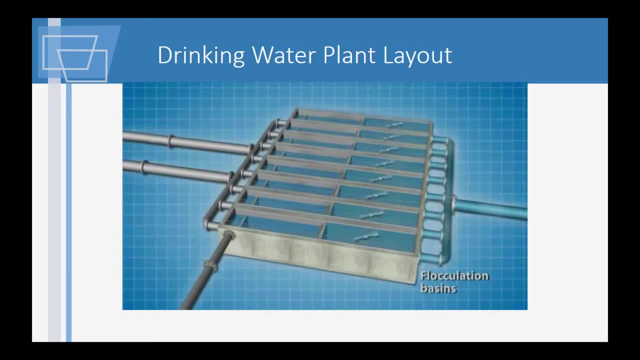 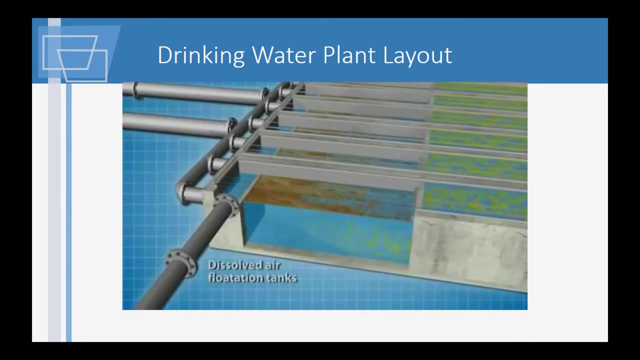 the particles to collide and stick together, creating large clumps. Now that large clumps have been formed in the water, the next step is to remove them. We do this in dissolved air flotation tanks. We inject a stream of water supersaturated with air into the flocculated water which 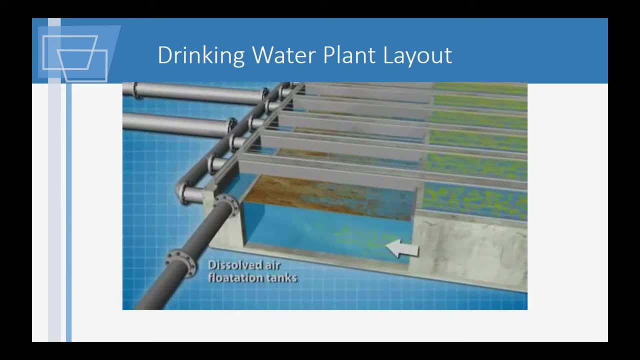 is flowing into the bottom of the tanks, Tiny air bubbles are released into the water and carry the clumps to the top of the tanks. Skimmers remove the floating clumps from the surface of the water. The clumps are pumped to an area for further processing. 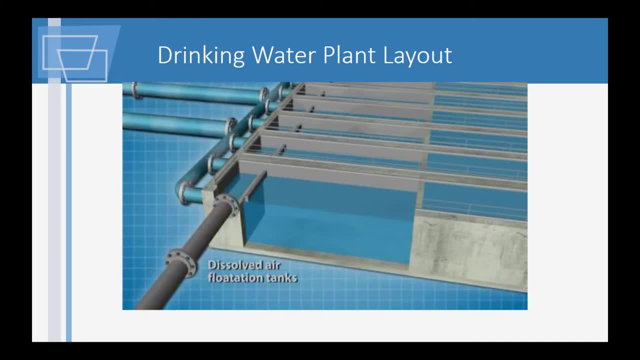 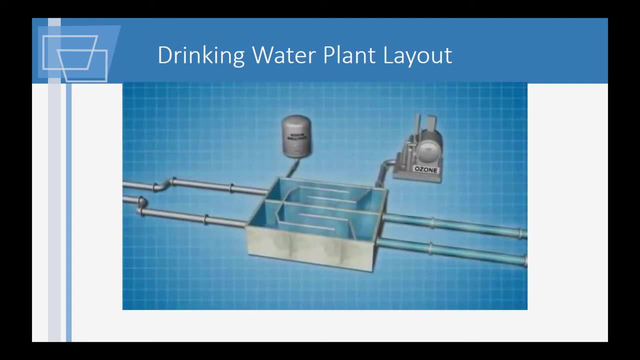 The treated water is collected from the bottom of the tanks. The water flows from the dissolved air flotation tanks to chambers where ozone is added. This step, called ozonation, does three things. It provides the first level of disinfection by destroying most of the harmful bacteria. 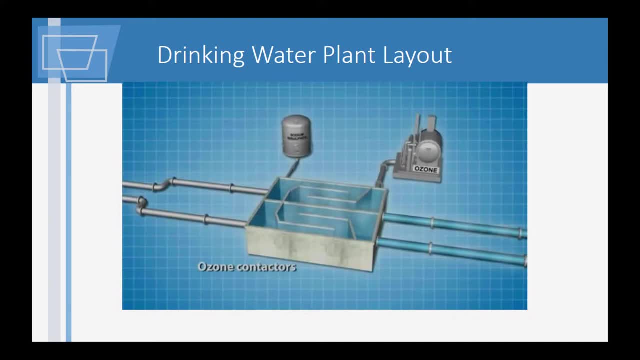 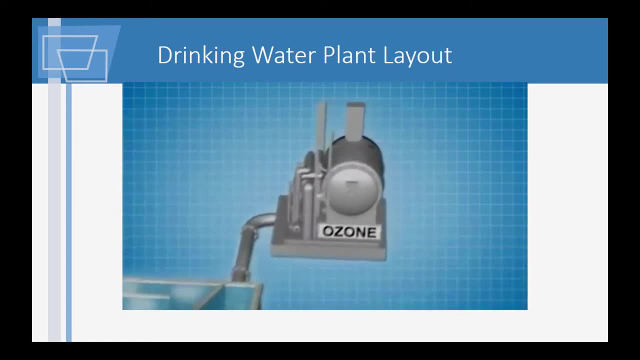 It improves the filter performance in the next treatment stage And it improves the taste and odor of the water. We make ozone by applying electricity to liquid oxygen. At the end of the ozone chambers we add sodium bisulfite to the ozonated water to remove any leftover ozone. 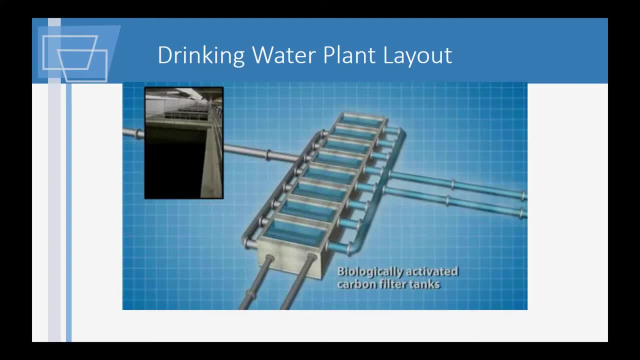 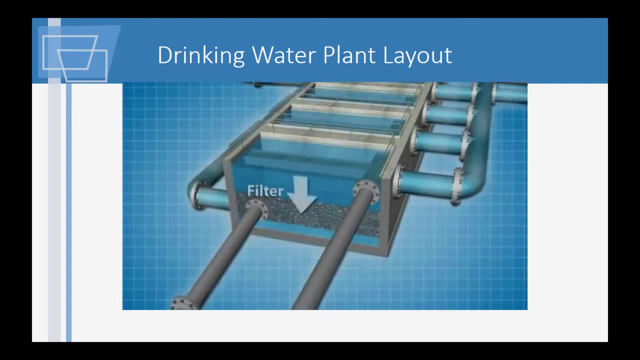 The water now flows into filter tanks containing biologically activated carbon. The filters remove any remaining small particles in the water, including parasites. Good bacteria growing on the filters removes some of the remaining dissolved organic material. This reduces the level of disinfection byproducts in the water. 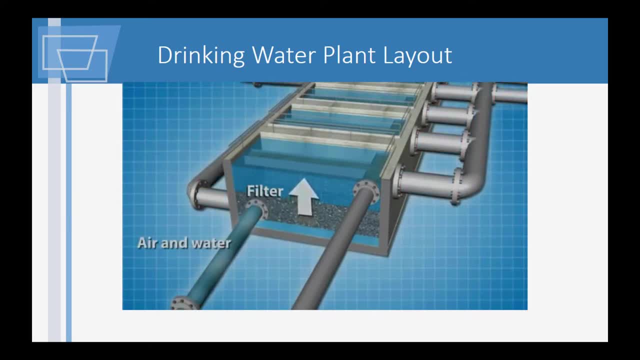 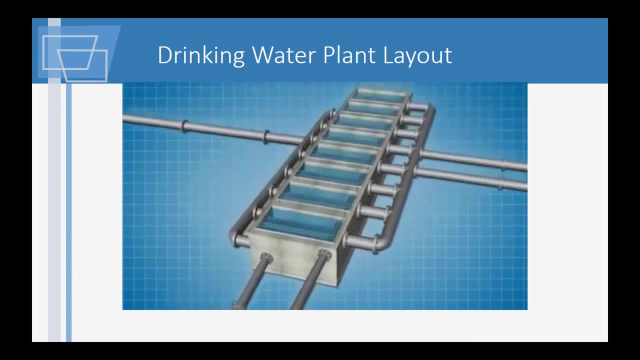 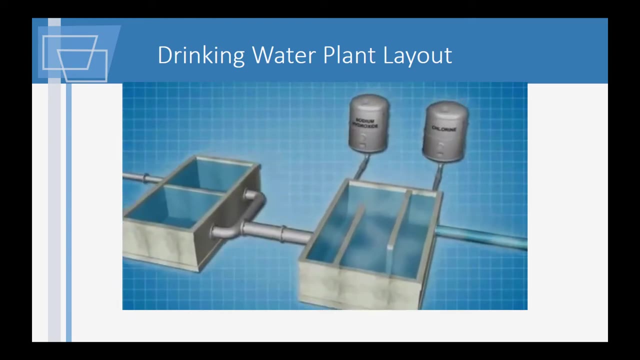 We clean the filters regularly by pumping air and water backwards through them. The backwashed water is pumped to an area for additional processing. The filtered water flows into the chlorine contact chamber for a second round of disinfection. We add chlorine to kill viruses and bacteria such as E coli that might be in the water. 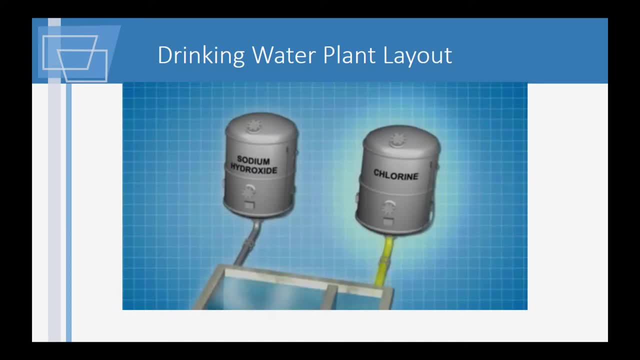 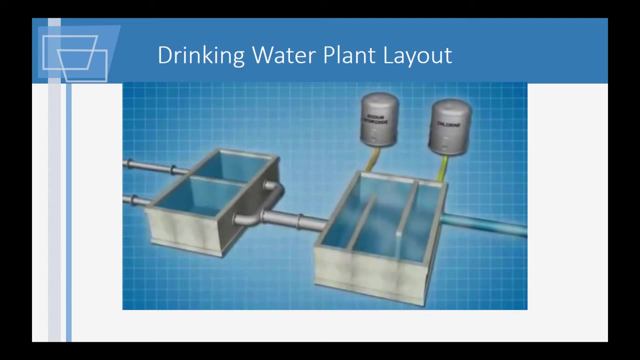 Chlorine is the most widely used drinking water disinfectant in North America and has been used for more than a hundred years. We then add sodium hydroxide to bring back the pH of the water close to the original level. The water flows from the chlorine contact chamber into an underground reservoir called the chlorine contact chamber. 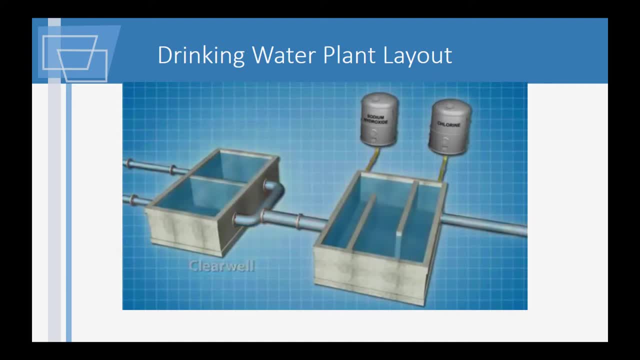 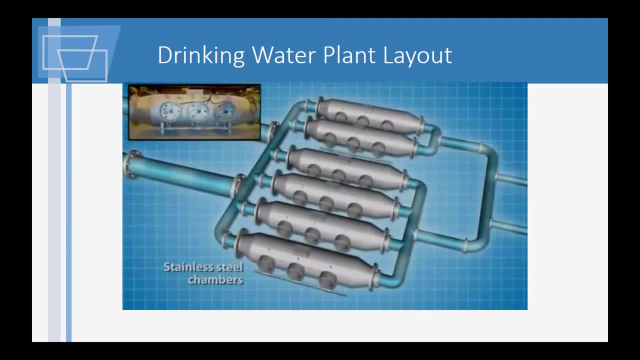 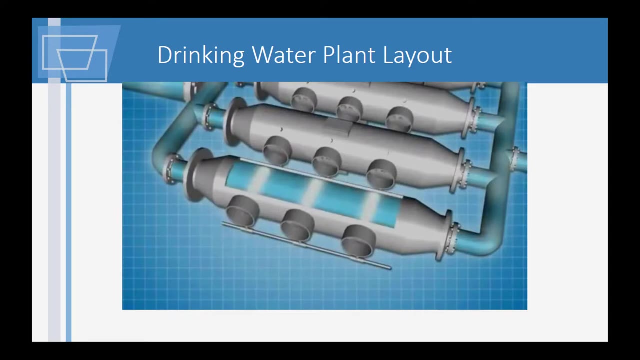 We disinfect the water once again using ultraviolet or UV light. We pump the water through six stainless steel chambers, each containing nine ultraviolet lamps. The lamps are similar to fluorescent bulbs, With only seconds of exposure. the UV light rays penetrate any remaining parasites, such as Cryptosporidium or Giardia. 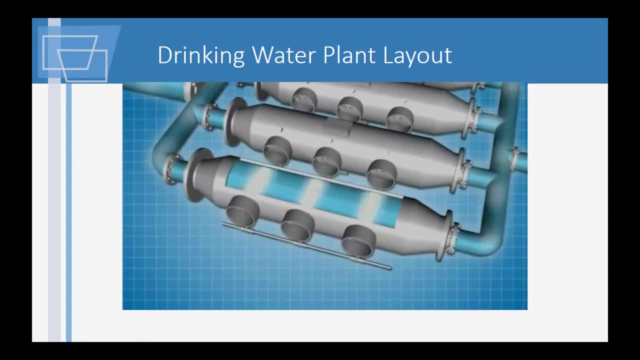 The UV light renders these parasites as if they were in the water. The UV light is then used to detect any other parasites, such as Cryptosporidium or Giardia. The UV light renders these parasites as if they were in the water. 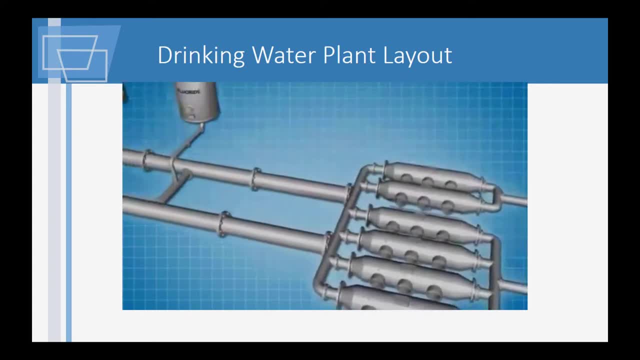 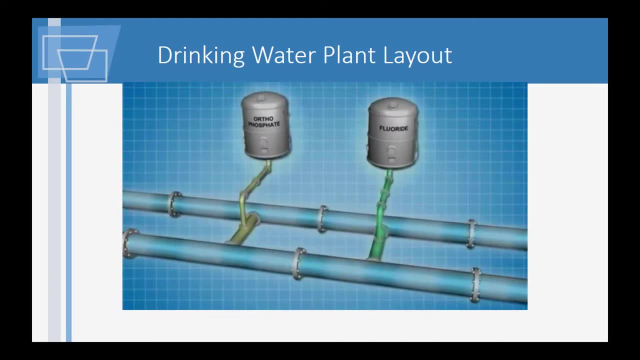 The UV light renders these parasites as if they were in the water. After UV disinfection, the water flows into two large pipes where we add fluoride to help prevent tooth decay. We also add orthophosphate to form a protective coating inside water pipes. 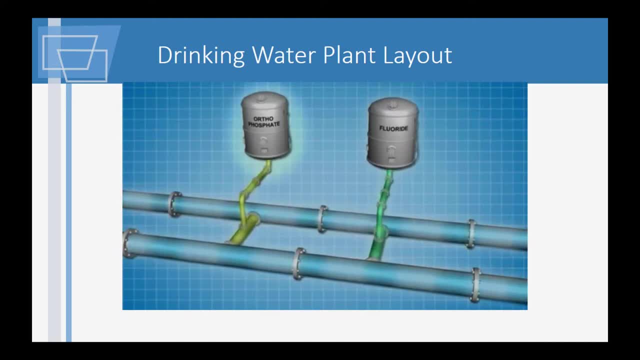 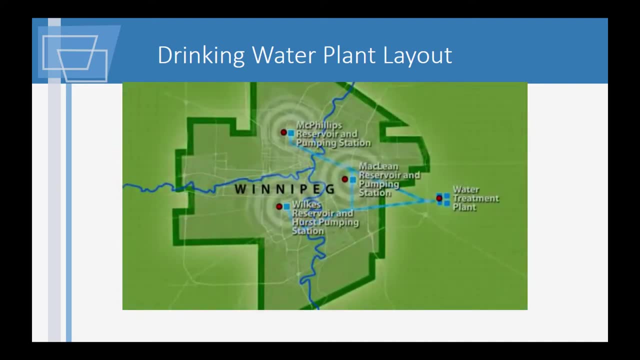 This coating helps reduce corrosion that may add lead to tap water. The two large pipes carry the treated water to our three reservoirs and pumping stations in the city. We add chlorine again as the water is pumped into the distribution system. We add chlorine again as the water is pumped into the distribution system. 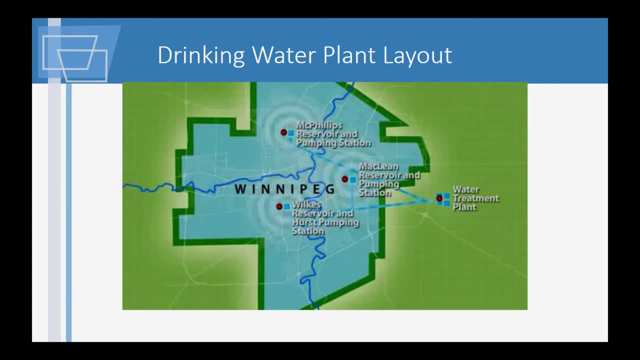 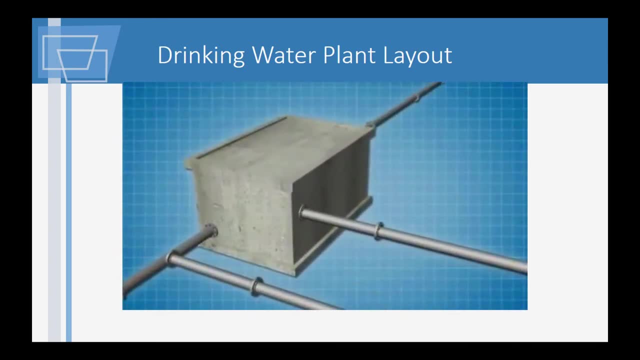 to ensure that the water remains disinfected until it reaches your tap. The final stage of treatment is to deal with the materials removed from the water by the treatment processes. The backwash water from the filters is allowed to stand until the solid materials settle. 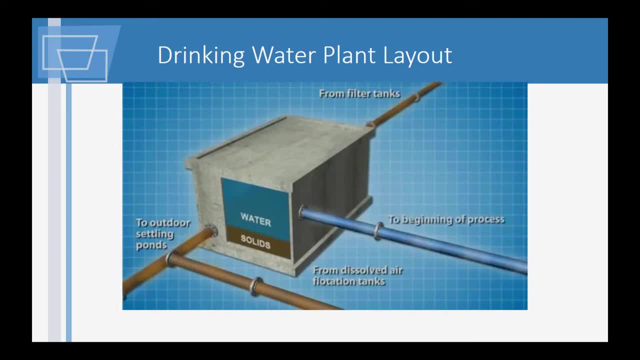 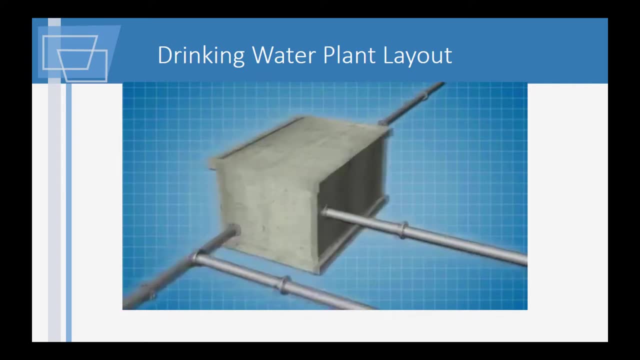 We then send the clean water back to the beginning of the treatment process. We pump the settled out material from the filters and the clumps of particles from the dissolved air flotation process. We pump the settled out material from the filters and the clumps of particles from the dissolved air flotation process. 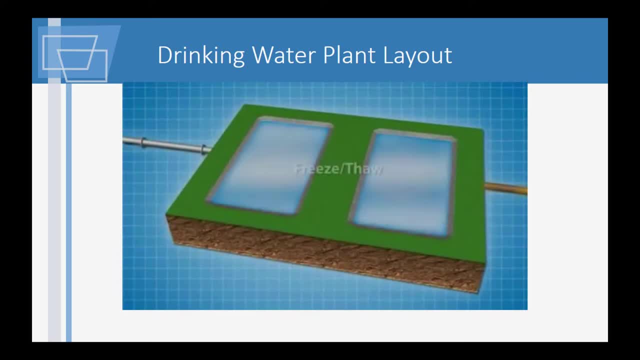 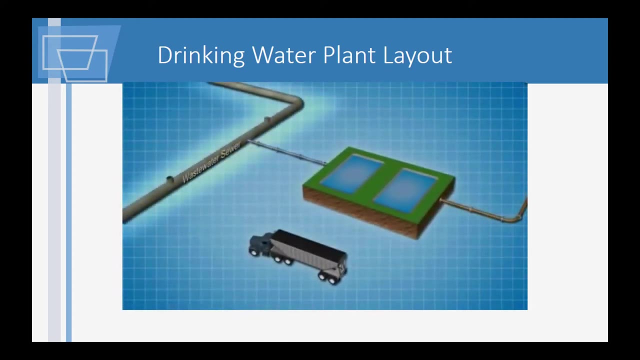 to outdoor settling ponds next to the treatment plant. The pond contents go through natural freeze-thaw cycles which separate the liquid and solids. The pond contents go through natural freeze-thaw cycles which separate the liquid and solids. We pump the liquid into Winnipeg's sewer system for wastewater treatment. 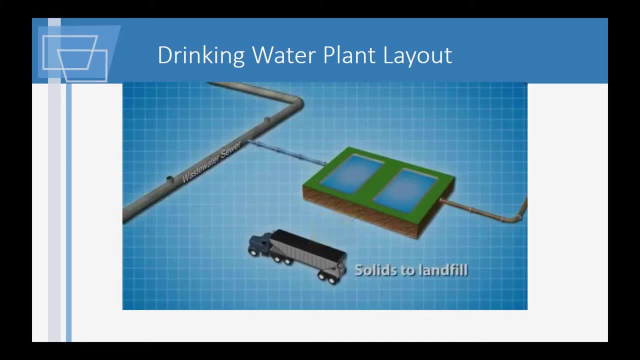 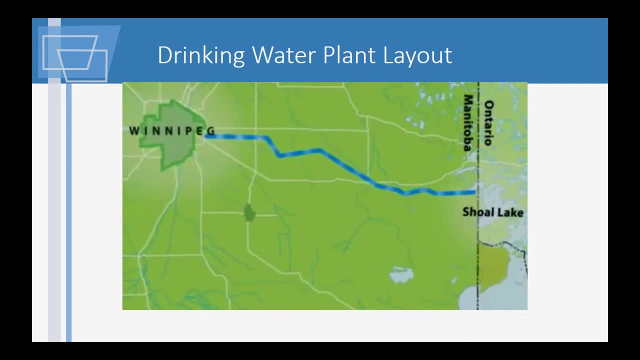 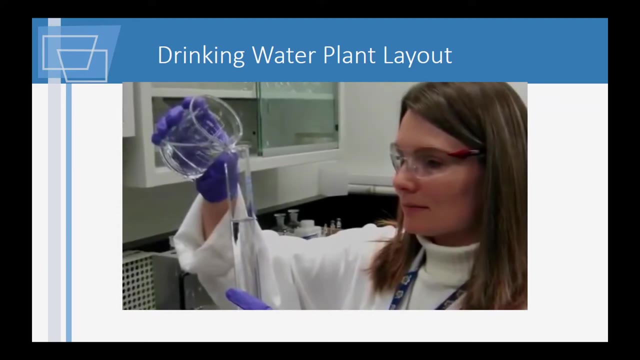 and take the solids to the landfill for disposal. and take the solids to the landfill for disposal. We test our water each step of the way from Shoal Lake to your tap. Our testing program includes over 150 different tests at more than 130 different locations throughout the year. 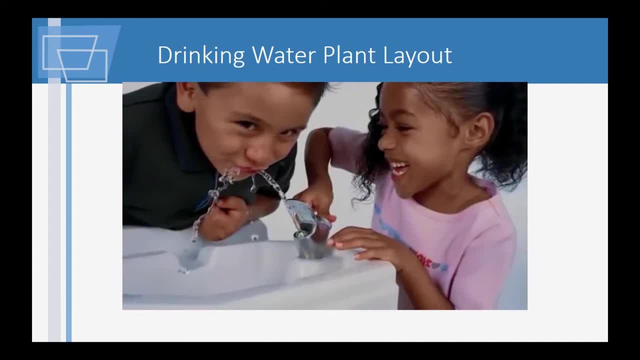 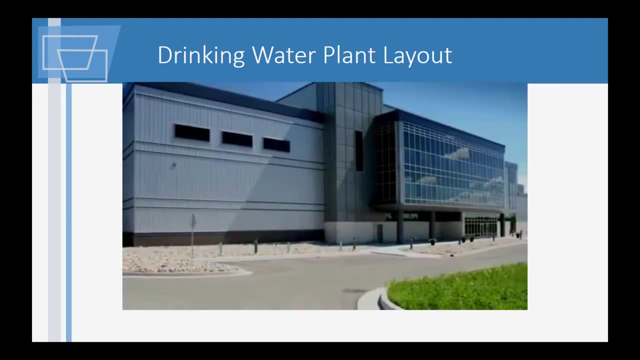 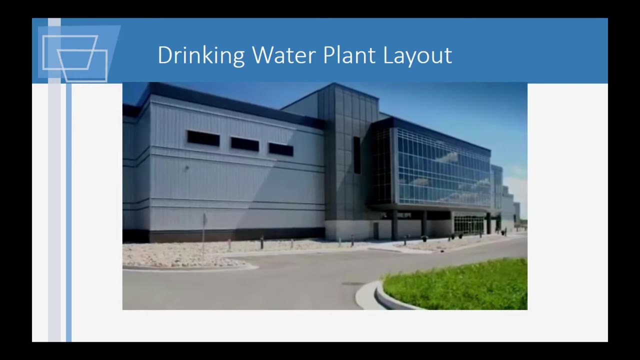 Because water quality is so important, we do more testing than the provincial government requires. Our certified professional team is dedicated to ensuring that our community enjoys safe, high-quality drinking water that meets provincial regulatory requirements and falls well within Health Canada guidelines. We hope that you've enjoyed this tour of our drinking water supply and treatment system. 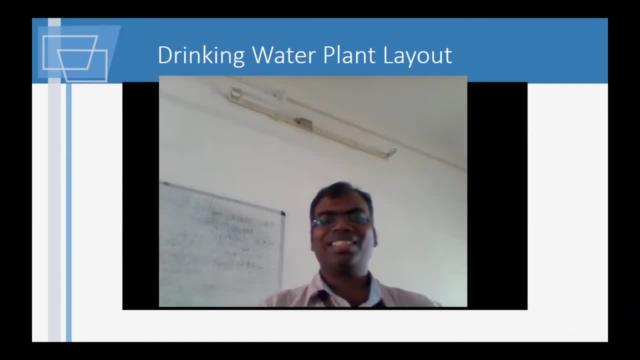 We hope that you've enjoyed this tour of our drinking water supply and treatment system. Great, So that was another drinking water system. What is unique about this plant? There is a disinfection after the treatment. Okay, And they are using the waste. they don't pay the water to the plant. 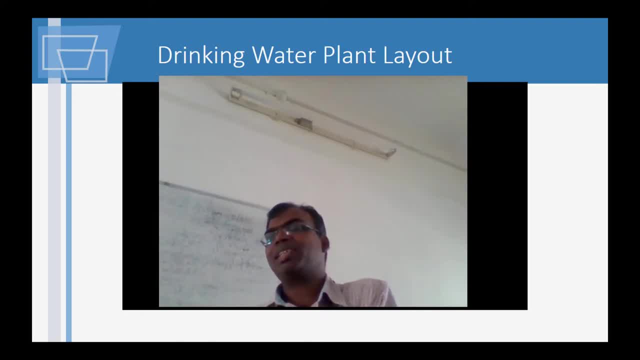 And they are using the waste. they don't pay the water to the plant. It's with the water. they don't use the waste. Okay, Okay, they add after the phosphate. Okay, They add after the phosphate. Why do they add it? 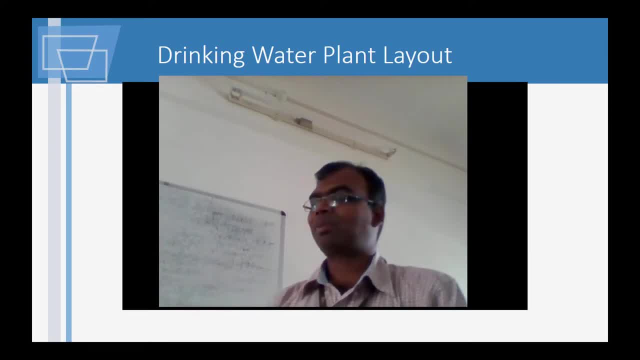 Because they couldn't have corrosion in the pipe. Because they couldn't have corrosion in the pipe, That's right. What about you, Nikhil? They add chlorination and ozone to the water. Yes, So sterilization is much more in this. 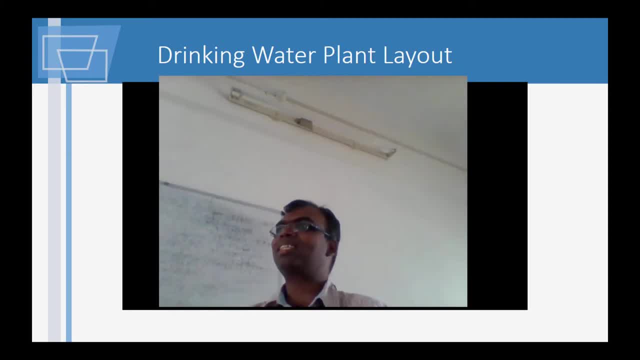 Okay. So first thing is, please note that in this video, in this tour, they showed some more about the way they conditioned water. for each stage, There was a pre-treatment. Sulfuric acid was added for some reason. Okay, this video again, this presentation is again coming to you. Okay, so why did they add sulfuric acid? Have a look at it. So all these other things which you told, have a look why they did it. Okay, so this is the most important thing, which I feel was a difference between this treatment plant or others. 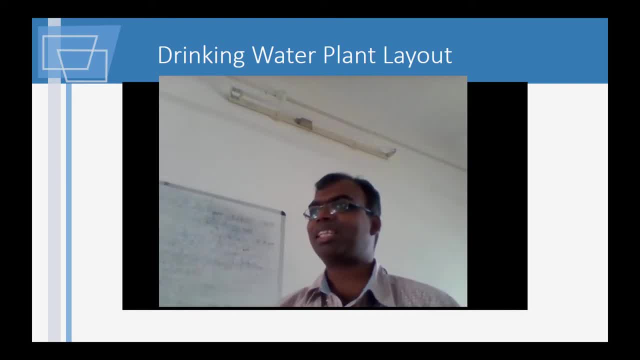 And they also talked about the sludge handling in this. Till now, in all the other videos which you saw, nobody spoke about the way the sludge was being handled. Okay, so this is something which is interesting and, in fact, much more than whatever I would have spoken. these people have given it all. I am not going to repeat what they told, but this short 10 minute or whatever was the length of that video. it conveyed much more of information than what I would have been able to pack in maybe 2 weeks or 3 weeks. 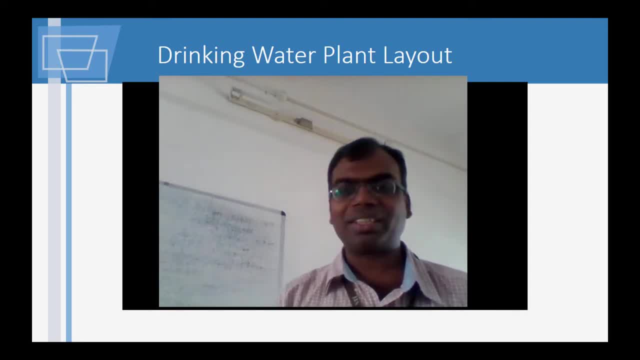 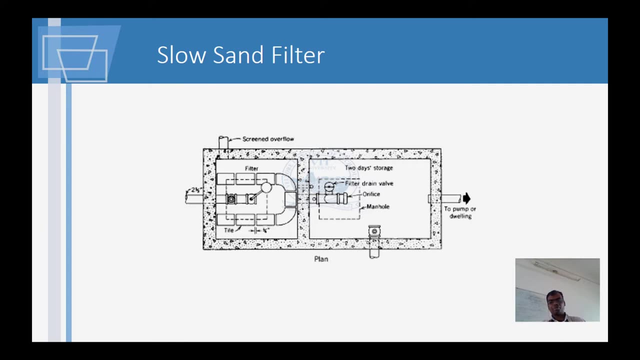 Because this is such a huge topic. basically, Okay, I am not worried about you guys, Because I know you are able to have a look at this and just try to understand what is there. I am going in for couple of layouts. Okay, Now suppose I am asking about slow sand filter, For instance. I want a diagram like this, indicating the main parts. 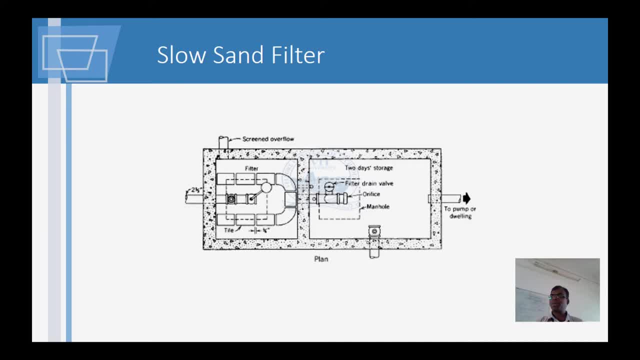 Okay, what is there, what is not there? Okay. so the more information you draw in a diagram, the idea of what is there, Okay. so the more information you draw in a diagram, the idea of what is there, Okay. so the more information you draw in a diagram, the idea of what is there. 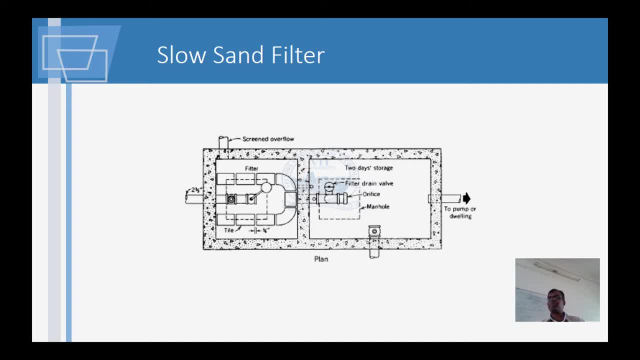 you got about. that system is very clearly indicated And when you write also, it will be ideal that you write point wise So that I know if you are writing something wrong. I will know it immediately even if you are writing the correcting. it will be easier for. 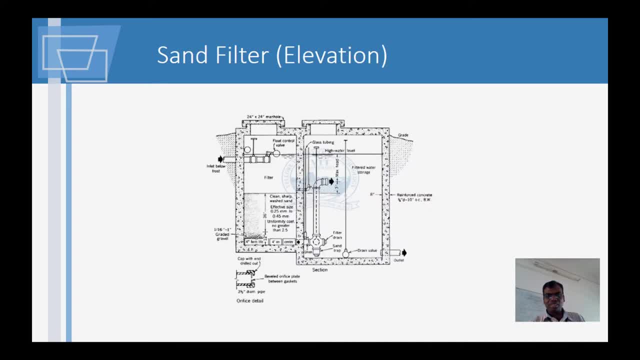 me to gauge your understanding. ok, So this will be the cross section and this will be the elevation of this. Now you just have a look at it. what is coming in through the pipe on a left? it comes in and then it forms a head over the filter bed. ok, There is a. 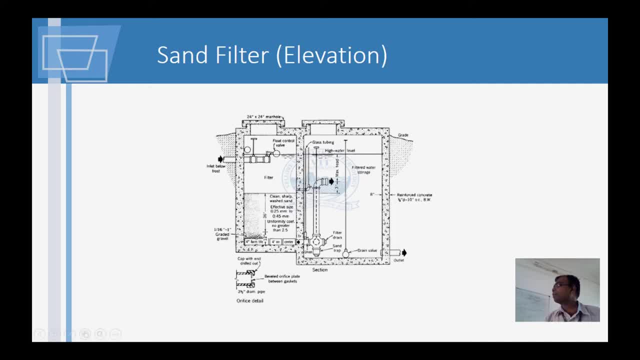 filter bed. there is a line over here, So this line is the place where the sand filter starts. and then, coming down a little, you will notice that there is a gravel bed. This is what you call, as they put it, as graded gravel. So this is the gravel bed. So this is the gravel bed. So this is the gravel bed. So 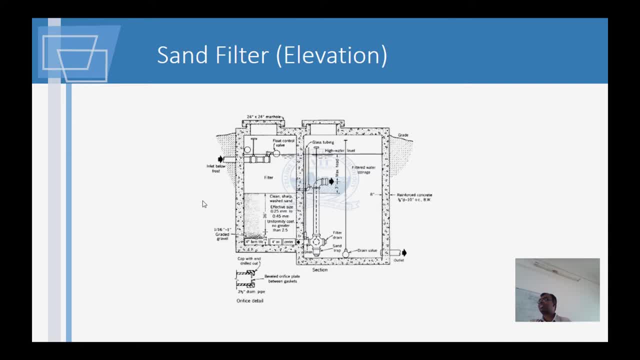 that means the particle. the gravel size will start from a smaller size at top. then it will be increasing in size. This gravel will be very important in letting the water flow through the water to the filter media. this is very much important- And then it will be collected. 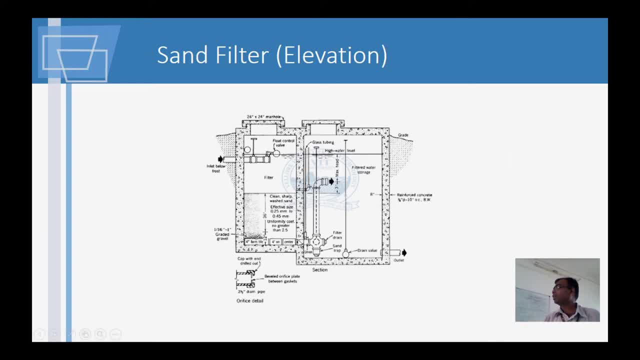 in this infiltration area, a pipe, and then it goes to the collection tank. So basically, see, this gives you a very clear picture of the sand filter. this is what we need. is anything else required? probably a backwash arrangement. ok, so apart from that, you don't, you don't. 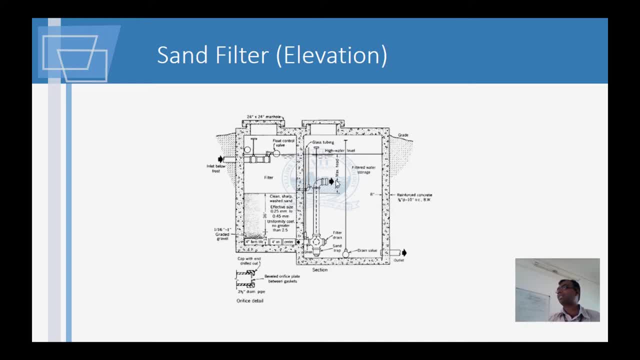 have. the whole thing is clearly explained, or it seems that you have to backwash nothing. there is another pipe, we just pour water through it. it will go in the water going through pressure and then it can go out. ok, so that's, that's the, that's the bag, that's what we have is. 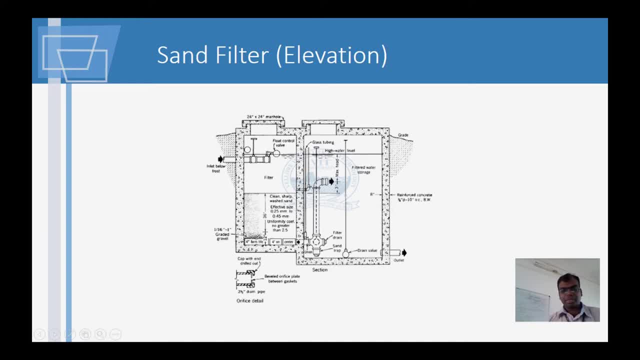 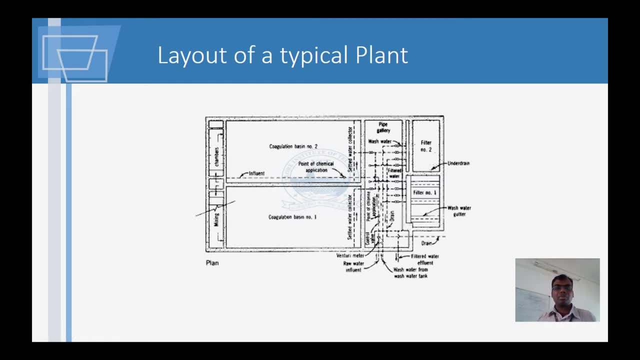 the backwash arrangement. ok, now the next slide i have is a typical layout of a plant. so entire plant has been put here. ok, so this is coagulation, basin one, coagulation. so i'm sorry i'm finding on computer coagulation basin number one. coagulation. basin number two: filter number one, filter. 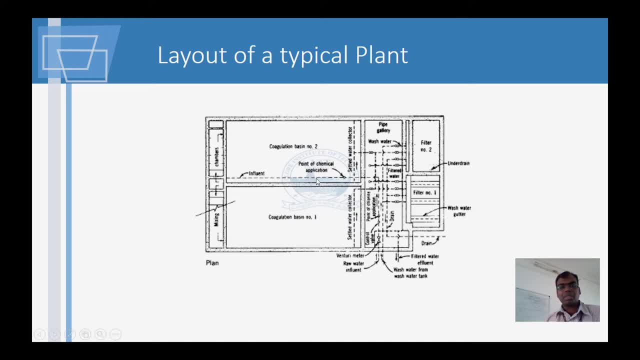 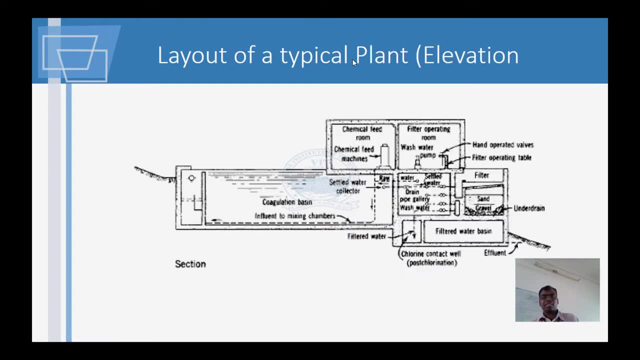 number two: ok, drain etc is all marked here. ok, so this is. this has been taken from a textbook. again, here you are having a cross section of the coagulation, of the coagulation basin, and then we got a chemical feed area and then filter. operating room: ok, of course you need a room. 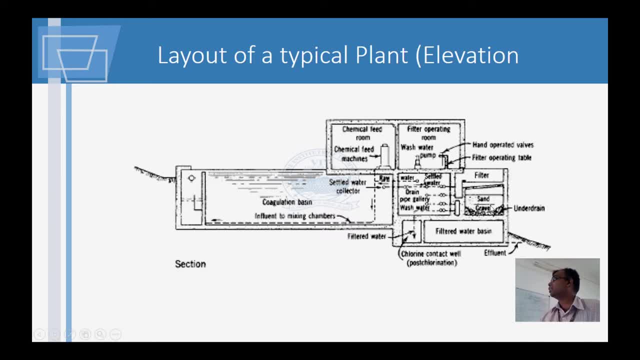 to operate the entire thing. and filtered water basin. it's stored at a lower level here, in the sense here there is a filter sand, is there ok? so it's a very basic layout and then it comes in, fills in here. this is a very, very basic because what happens is a very complicated layout. if you present on this one, it doesn't. 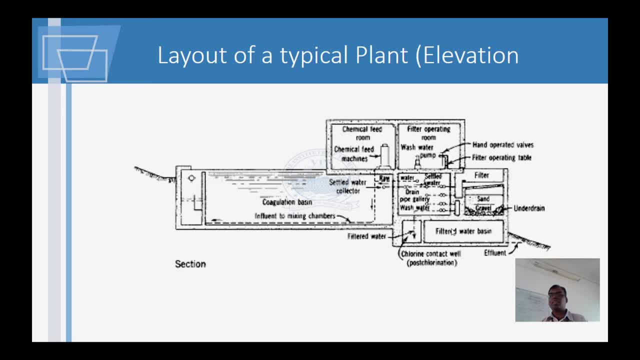 show up at all. i hope you're able to read what is there- the text. of course you'll be able to do it in your when you take the powerpoint presentation. you can probably zoom in and all that and see. so that's about this. this is my reference for much of my lecture today. 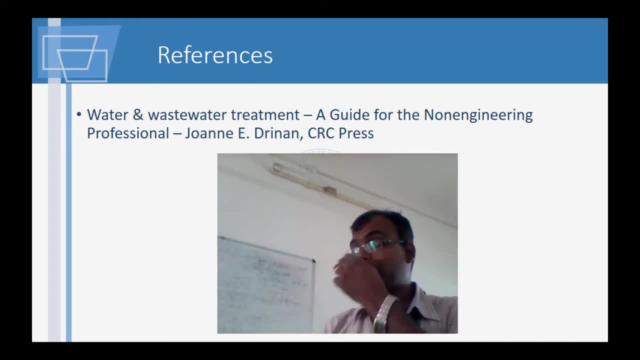 i hope you enjoyed it. this is a very basic. it was very good but very gentle ideas, doesn't go too much into the details, but I don't know whether you found it too basic. today's lecture, the principle, will not change across anything. be it sewage, be it drinking water, the process is the same as in aeration. is there? 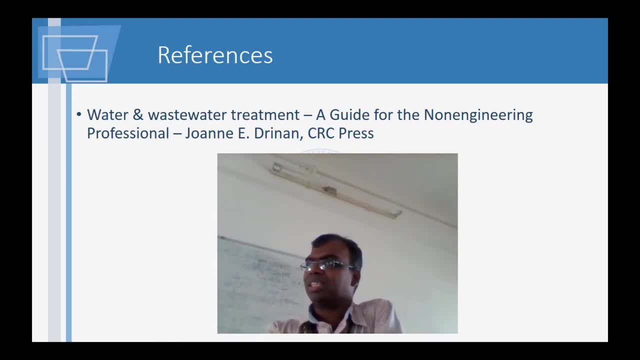 some mixing is there? what you mix in is what is different? yes, I'll just, since I showed the sand filter. okay, so in each of the processes which we talk about, each of the processes we talk about, there is a problem associated with it. okay, now, maybe, if you were talking about this in particular, this will be more relevant to a sewage treatment. 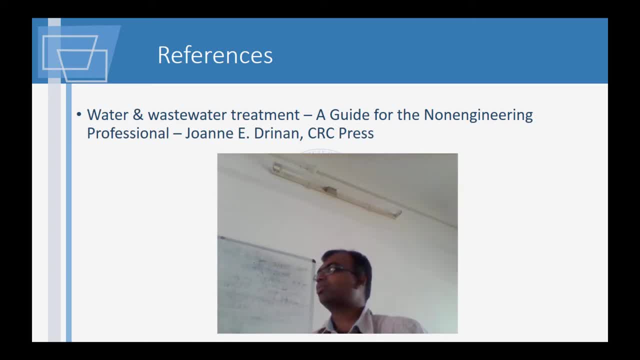 but I'll just put in a word, I mean I'll just add this: so what could be the problem in a sand filter clogging? then there is something there will be, there is a chance at. order is cost, because when water, whenever water is stagnates, you can have order problems. other thing is, it will stay. 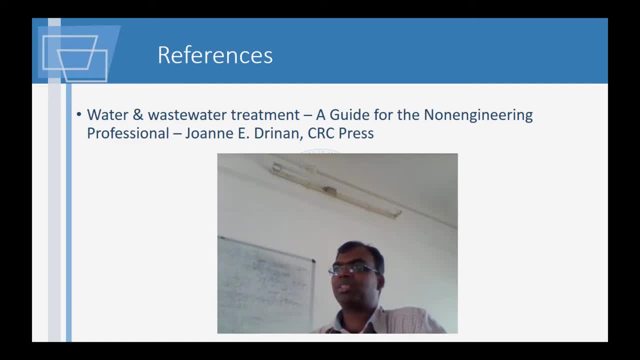 it will become a breeding. breeding the when problems will occur. okay, so it can. zombies usually: Если вahθσα реш väldigt的話 for mosquitoes and stuff like that. so I don't know whether it will be nice to go and spray pesticide on that water or not. then you can also have another thing. 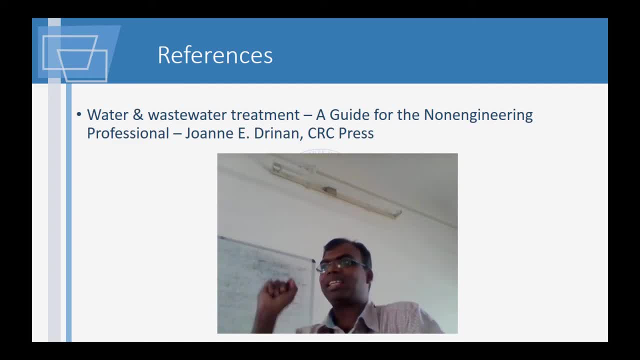 there's a very specific flight called psychotic flight that likes to go in for and it's it's a, it's a documented nuisance for this water treatment plants- psychotic flight. so these are some of the things which we can say is a problem with the operation of the sand filter. so you can always think about some things. 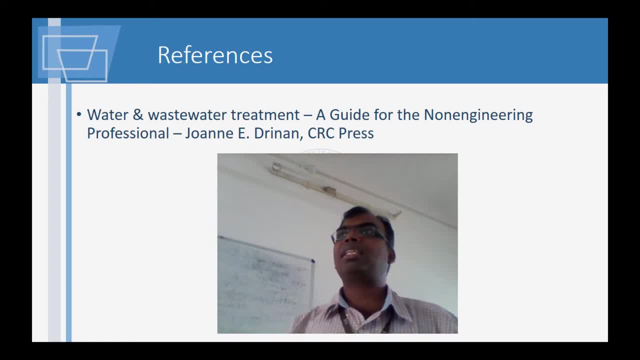 like: what is the problem associated with, let's say, coagulation basin? what could be the problem? think about it, you can write it down, okay. or even if, what is the filter media? same problem in clogging of filters. sometimes you will also find that certain the presence of certain chemicals, for instance zeolite process. 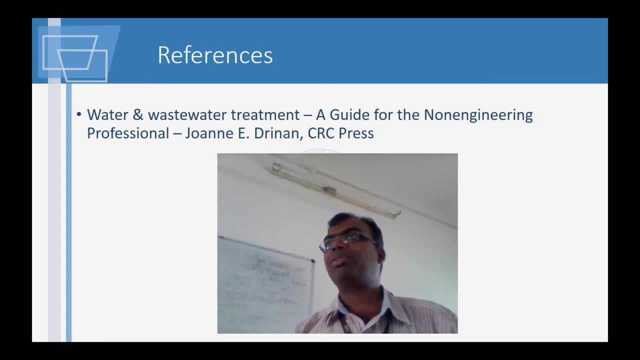 you cannot have certain chemicals in the water. if you have that, it will affect the zeolite membrane. what is that? so these sort of things will be required to be learned. it means just do a little bit of reading. widen your horizons. stick to, don't stick to one book. read the same thing in two or three books. okay, next. 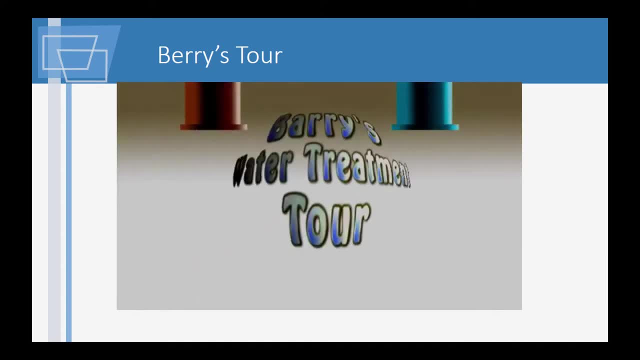 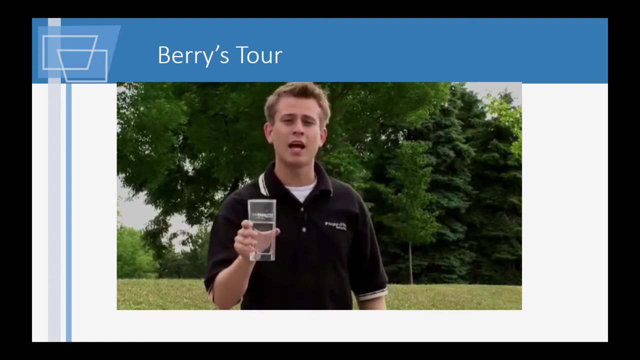 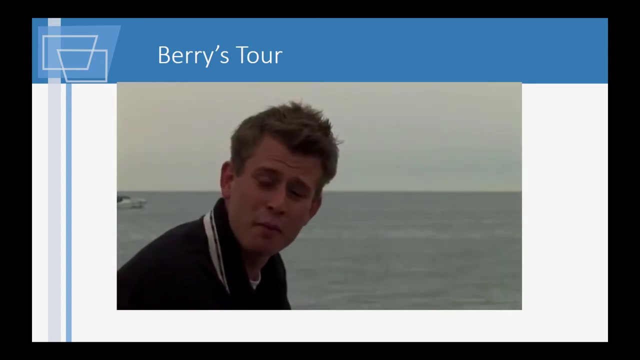 time. have you ever wonder where your water comes from when you turn on your tap? hi, my name is Barry, and today I'm going to show you how your water gets treated. the journey begins here at Lake Ontario. an intake pipe big enough to drive a car through extends two kilometers offshore and lies at the bottom of Lake Ontario. 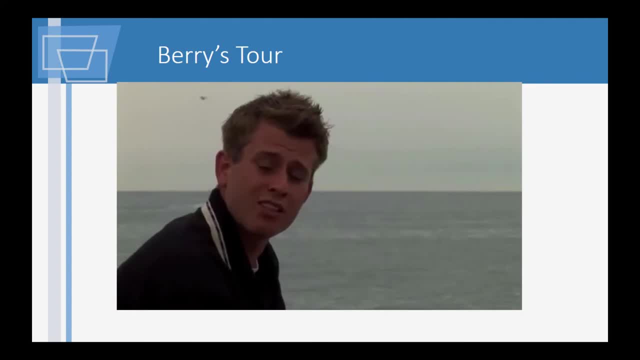 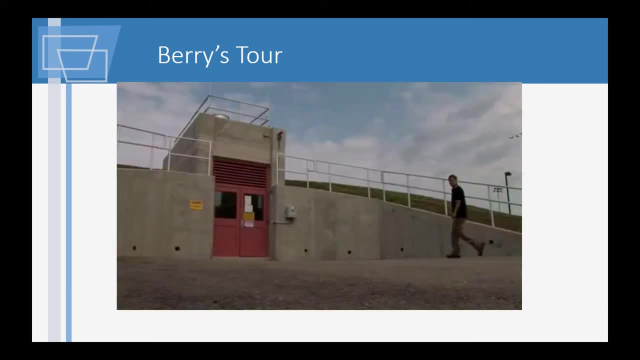 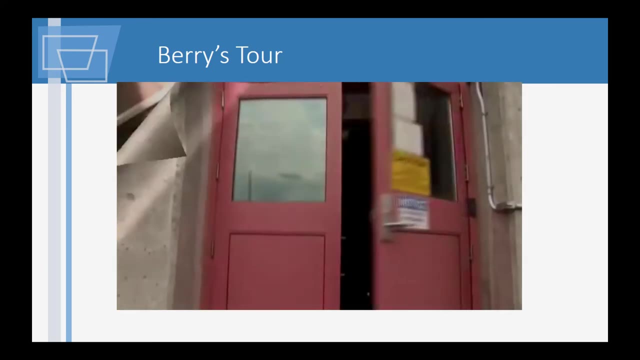 ten meters deep. the end of this pipe is covered by a screen to vent large pieces of debris from entering the water treatment facility. let's go there now. we're now at the facility. I'm going to show you each step of the water treatment process here. the water first enters the facility. every day we can 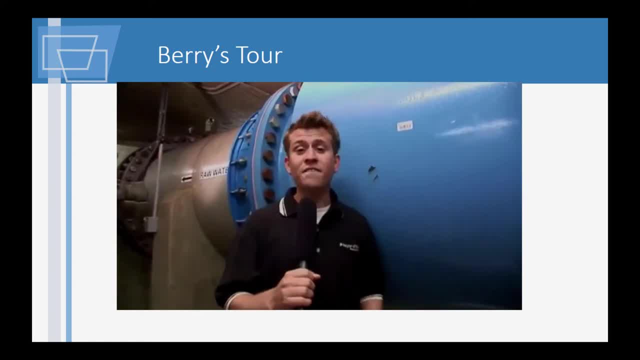 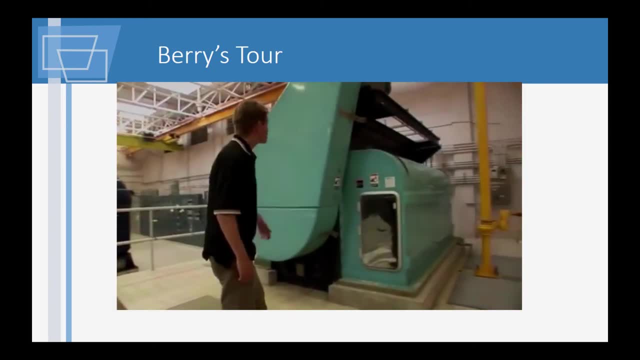 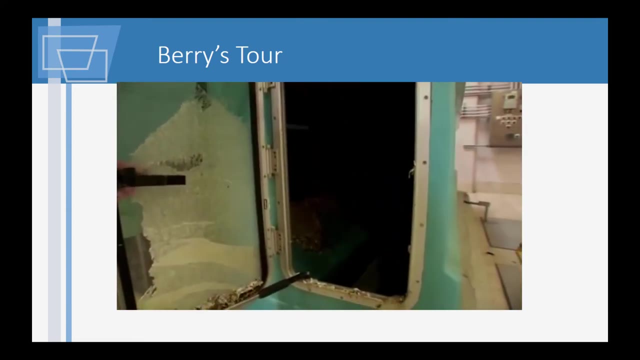 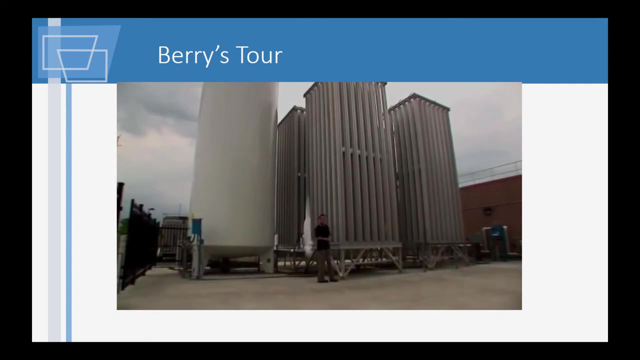 process up to 820 million litres of water that could fill up the 330 Olympic side swimming pools. inside the facility. the water flows through these traveling screen where a copper mesh has smaller items like fish and plant life from entering at the Lakeview water treatment facility. we turn oxygen into ozone, but first we 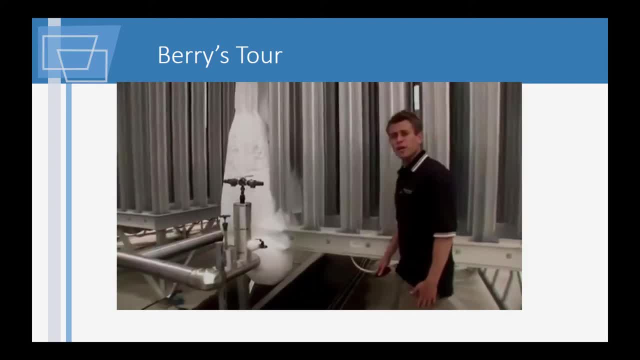 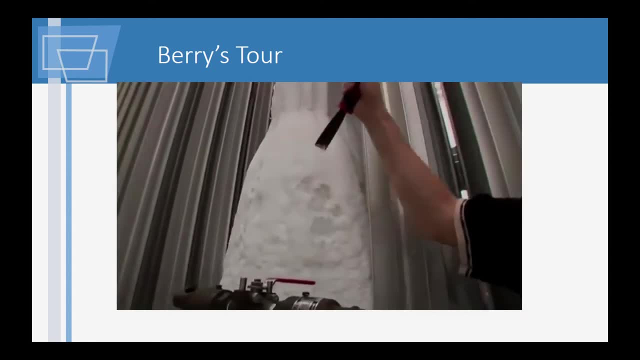 have to get the oxygen to our facility. the easiest way to transport oxygen is in liquid form. once it's here, we keep it cool in these large tanks, which is why ice forms, even on a summer day like today. We then transport the oxygen into our facility. 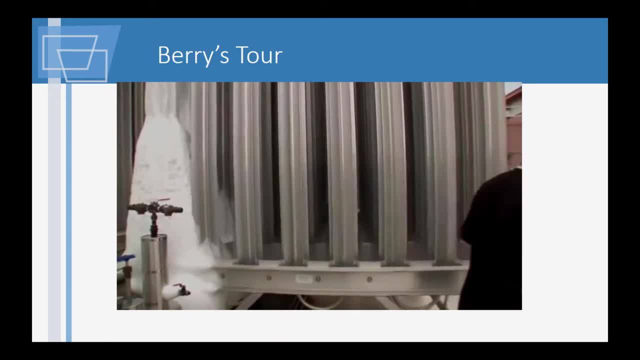 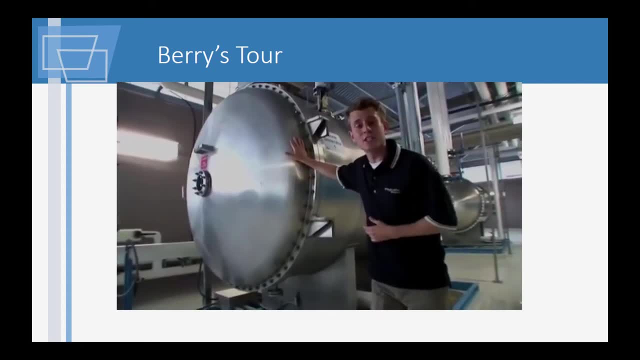 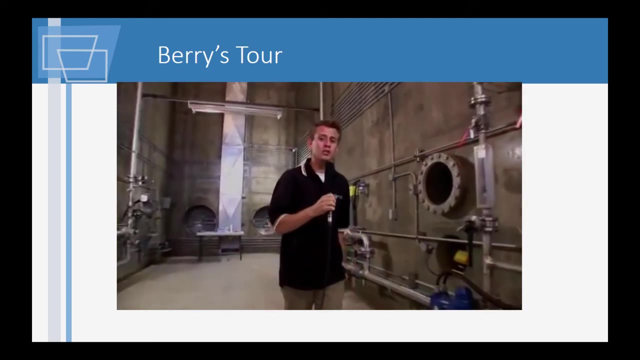 where it's converted into ozone. Let's go take a look. This is the ozone generator room. Inside this generator, an electrical current is passed through the liquid oxygen and converts it into ozone gas. Next we diffuse the ozone into the water as tiny bubbles. 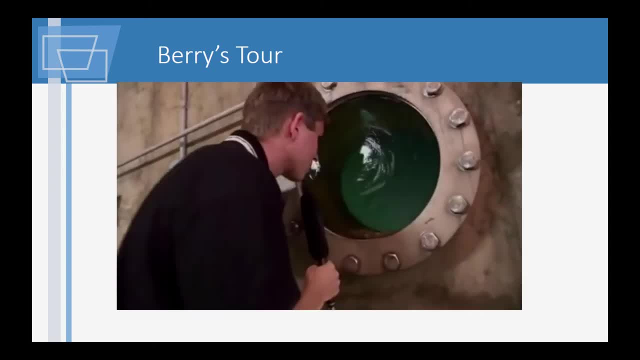 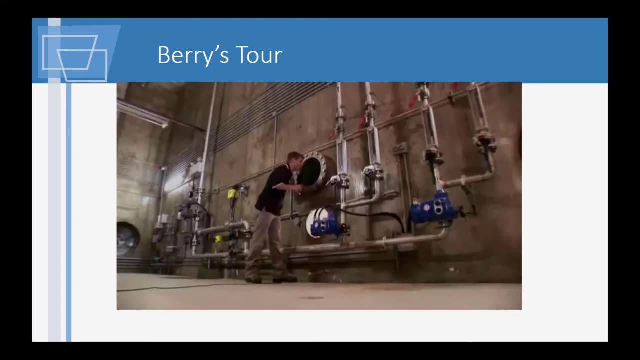 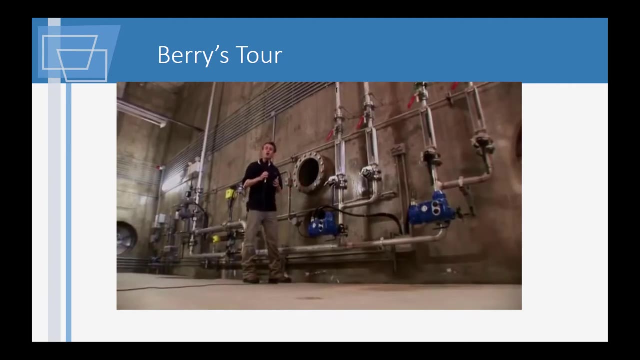 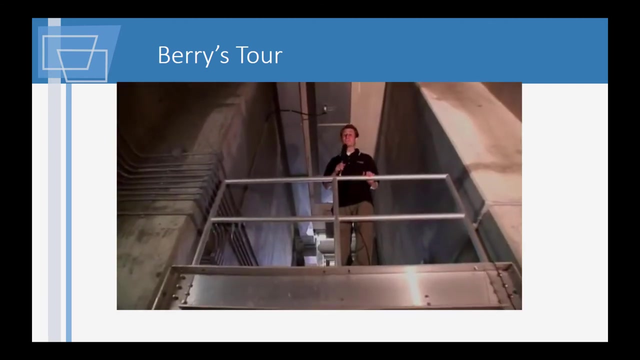 This is part of the disinfection process. The ozonated water remains in these large concrete tanks for 30 minutes before we add sodium bisulfate to quench or remove the ozone before the water moves on to the next step. This makes up the first step of the disinfection process. 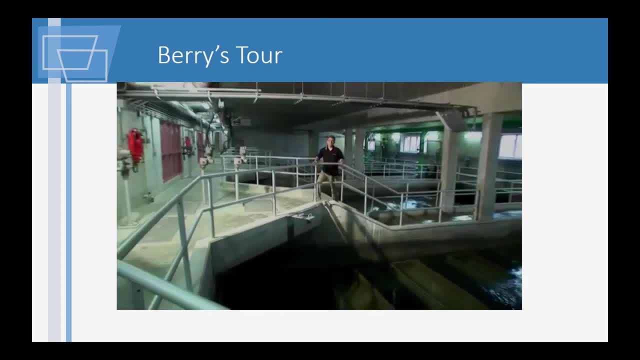 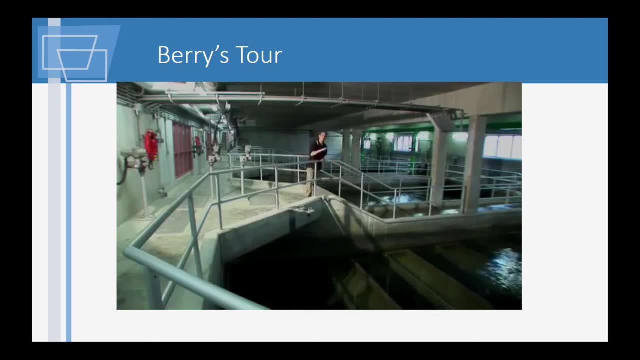 We'll now look at the next step in water treatment. The disinfected water flows from the ozone contactors to our biologically activated water. Here the water flows in from the top and filters through tiny pieces of carbon which have been heat treated and resemble the carbon. 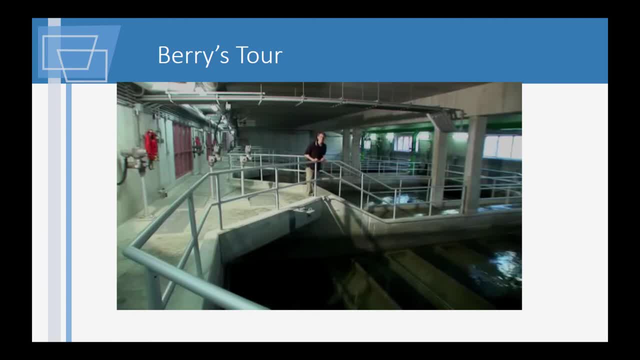 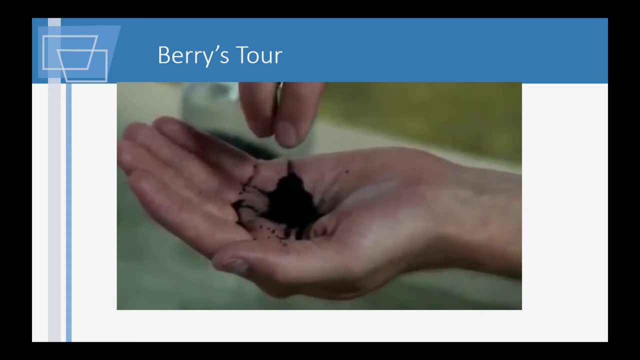 found in a home water filter. Harmless bacteria live in the crevices of these tiny carbon pieces. These bacteria consume the organic material broken up by the disinfection process. This step helps to remove a lot of the bad taste and odour from the water. 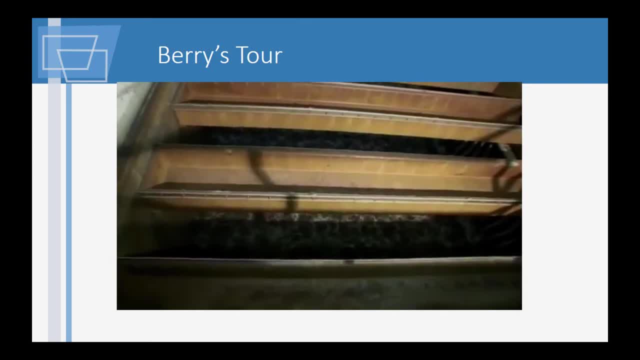 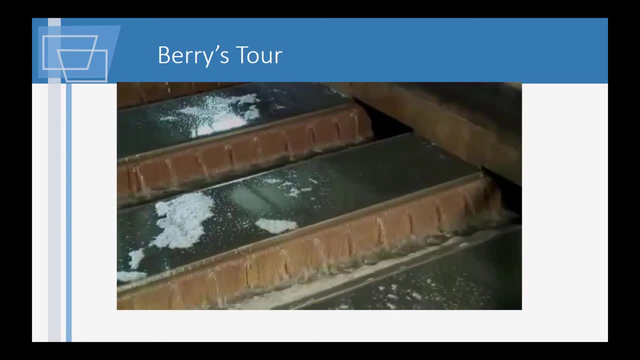 These tanks are five metres deep with over three metres of water in them. This is the first step. There's over three metres of biologically activated carbon at the bottom. Every five to seven days, these tanks are backwashed. Clean air and water are forced backwards through the system. 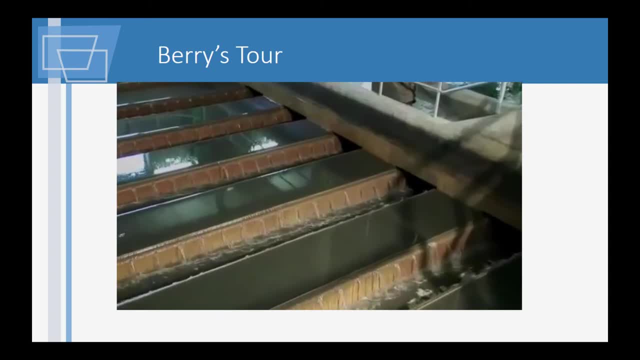 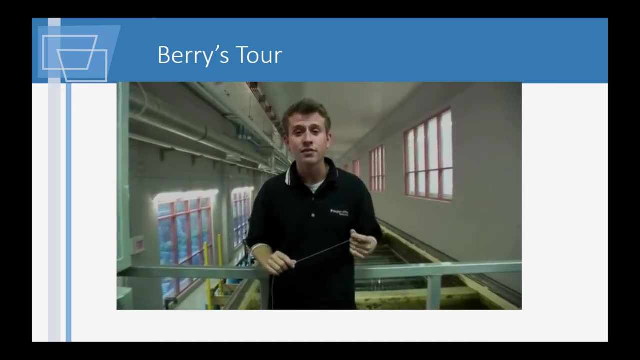 to break up and flush out anything stuck in the carbon. Next we'll look at the ultrafiltration membrane process. The water flows from the biologically activated carbon contactors to a series of filter membrane units. The units are made up of tiny membrane fibres like this: 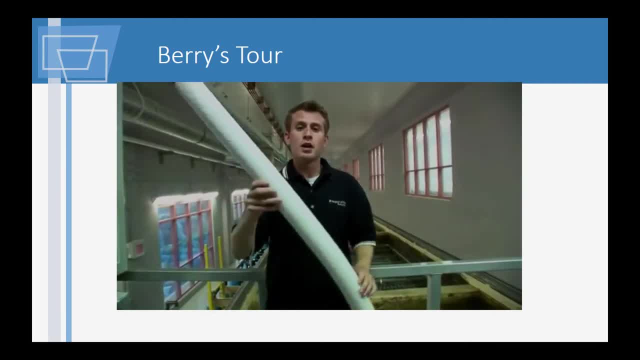 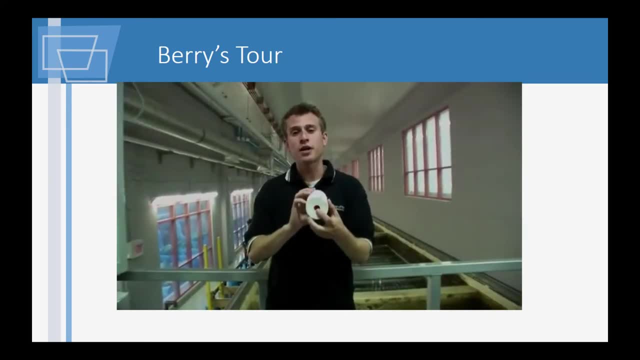 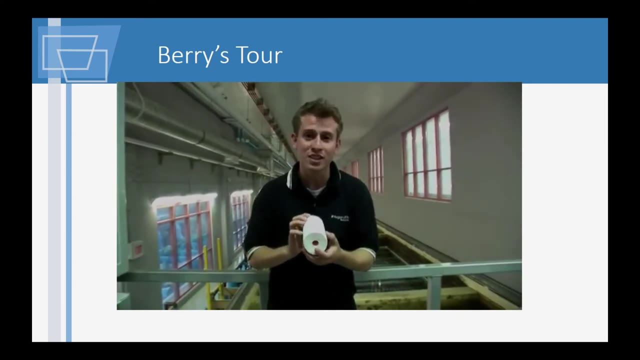 This is a model of a membrane. A membrane fibre is a tiny tube with millions of microscopic holes on the outside. We draw water into the tube using vacuum pressure. The holes are so small that only water can pass through, and pathogens, bacteria and particles are left on the outside. 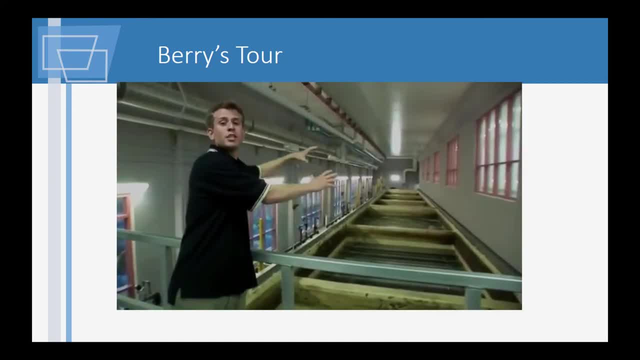 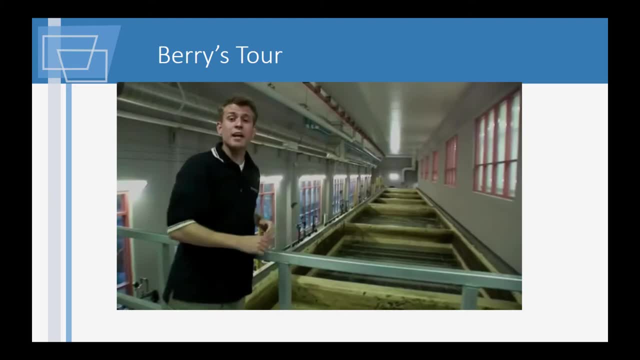 To filter the water on a large scale. we have 12 membrane trains, each holding 55,000 litres of water. Each train has 672 modules. That equals over 282 million membrane fibres. We lifted the cassette from the train. 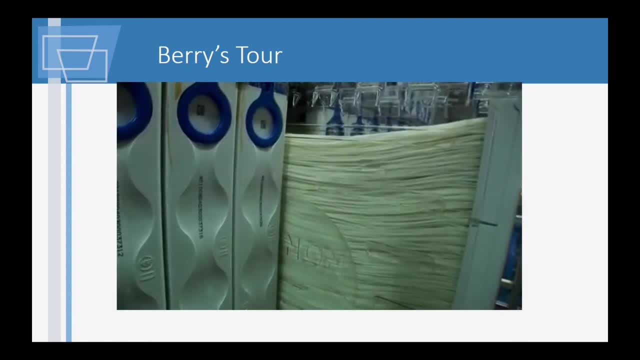 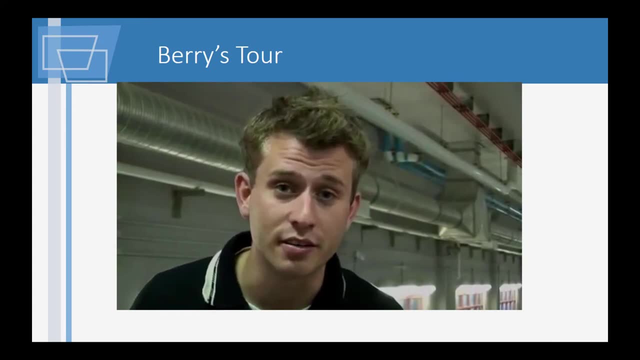 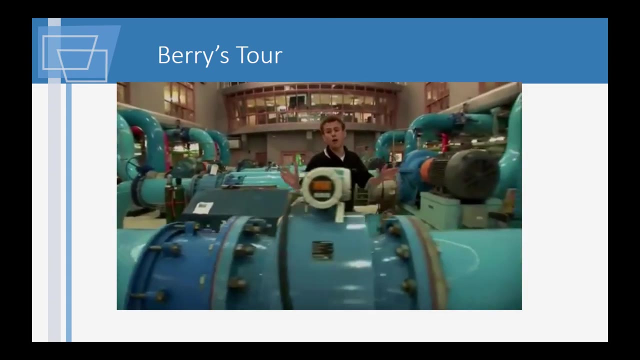 so now we can see. the fibres are grouped into modules. Each module is made up of 35,000 fibres. Now the water is clean and almost ready for distribution. These blue pipes collect the clean water from the membrane trains Before the water heads out to our reservoir. 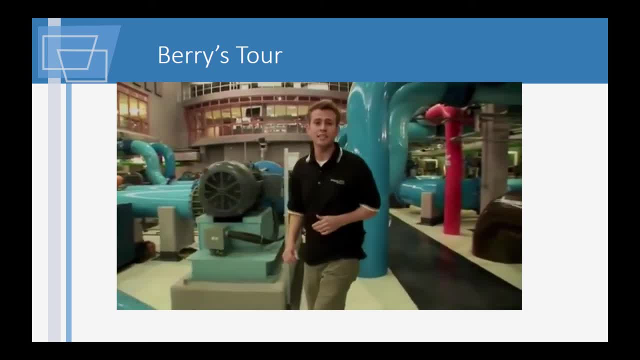 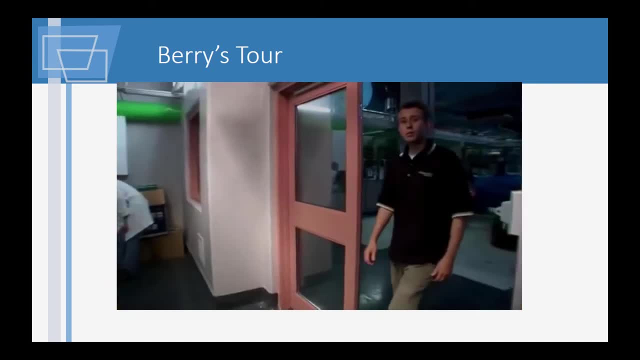 we add a small amount of chlorine to keep the water clean and disinfected as it heads over to your tap. We also add a small amount of fluoride to help promote dental health. As we prepare the water to leave the facility, we constantly monitor its quality. 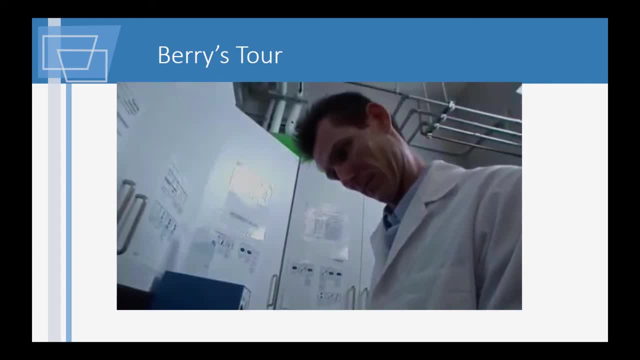 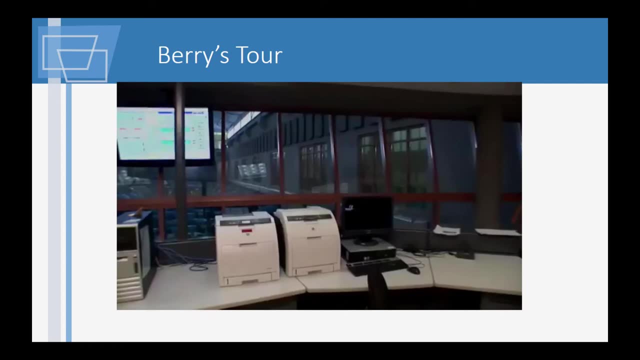 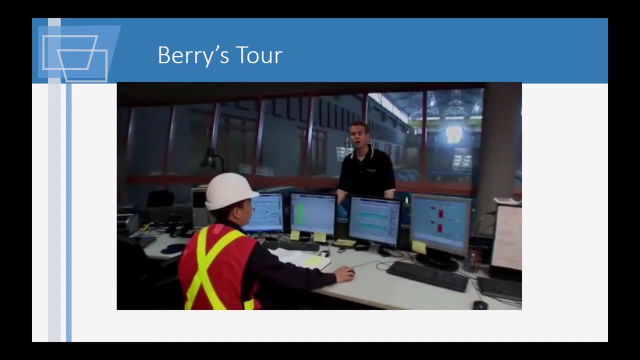 to ensure that it meets the Ministry of the Environment's stringent water quality standards. We also test the water manually four times a day for over 100 different parameters, And back here in the control rooms, our operators monitor the entire facility and each stage of the water treatment process. 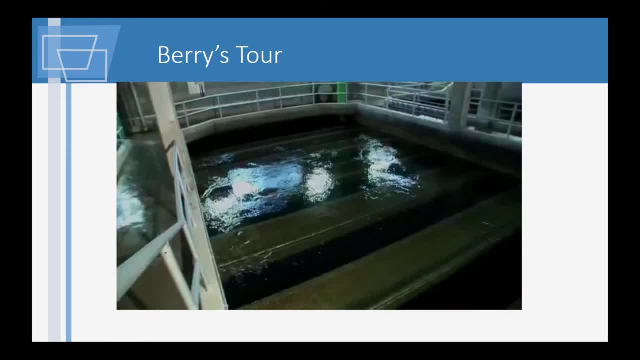 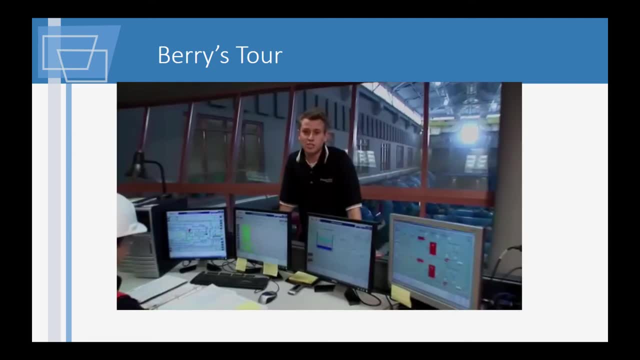 For example, they control the back washing that we saw in the biologically activated carbon contactor gallery, They ensure the membrane trains are functioning properly and they determine chemical dosages such as ozone. The blue pipes from the facility carry the clean water to an underground reservoir. 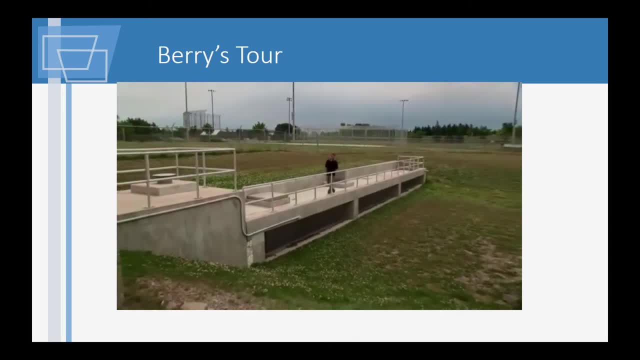 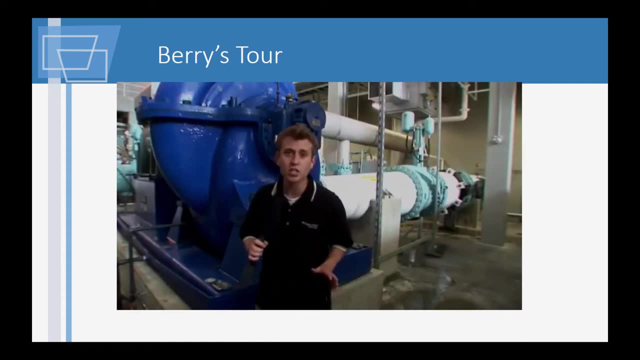 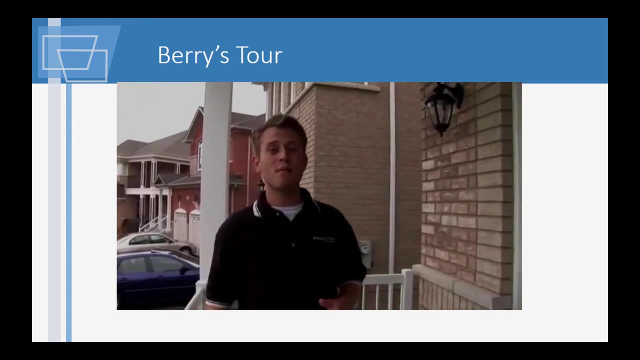 Reservoirs are huge storage tanks for water and are located all around Peel Region. Popping stations push the water out into a network of underground water mains that connect to your tap. Water treatment is a complicated process. It takes up to four days from the time the water leaves Lake Ontario. 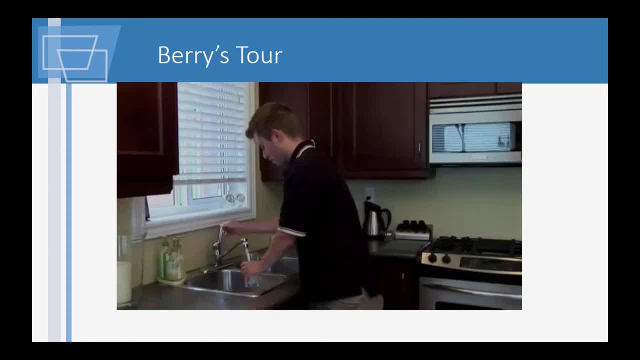 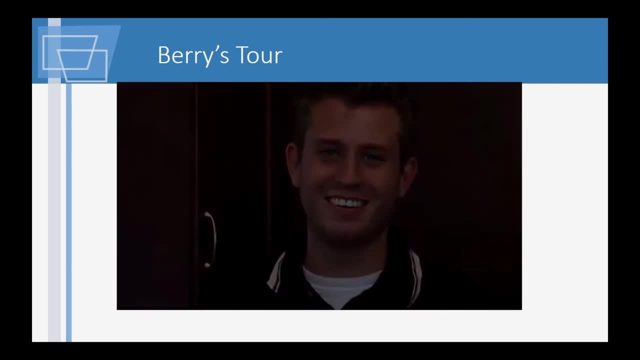 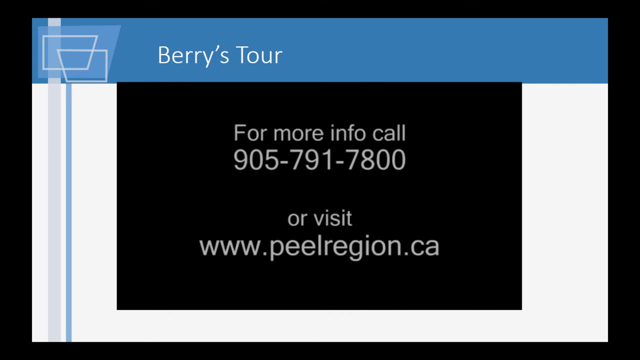 until it reaches your tap And it's ready to drink. For more information about water in Peel, contact us at 905-791-7800 or online at wwwpeelregionca. So both of these were something in Canada, Both these videos. 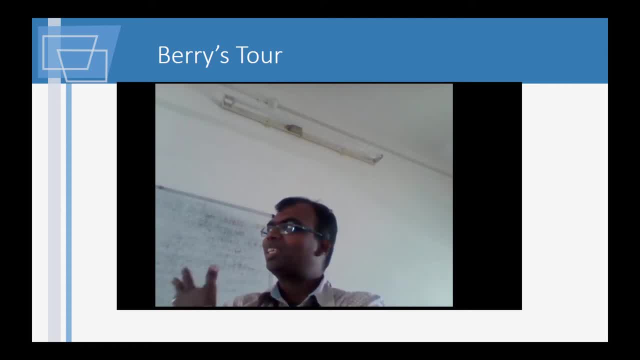 What do you feel about this treatment process? What was different here? Instead of Yes, They used membranes, Actually they did use filters. There was a sand filter at the beginning. Okay, Sand filters there, and activated carbon is also being used. 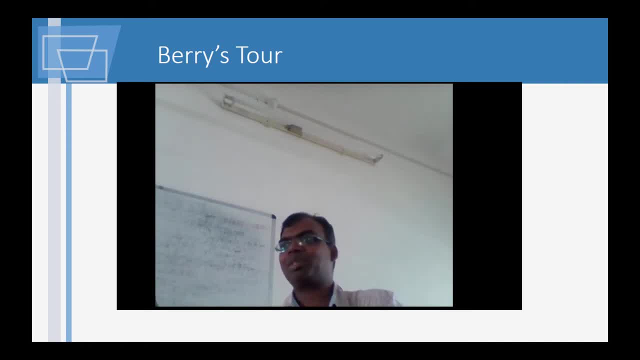 Okay, And in this one they didn't talk much about other filter, other things. There's not much talk about chlorine and what do you call UV? Yes, So membrane is such that nothing can pass through other than water. So this is what essentially happens in most of the reverse osmosis processes. 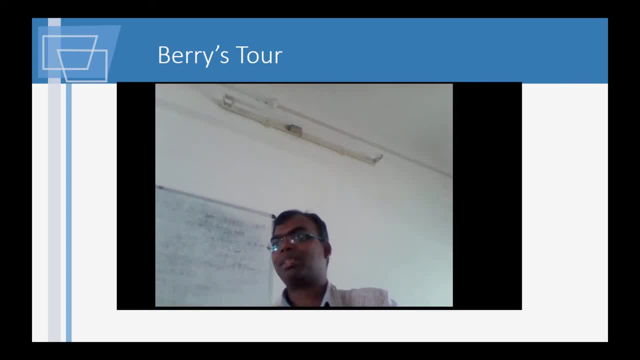 Here it might. it is ultrafiltration, But reverse osmosis is also concerned with membranes And please remember the principle that of underground storage is there in India also. If you look at those tanks, they're huge, very huge, And you will have to keep. it will look like a big ball with columns. 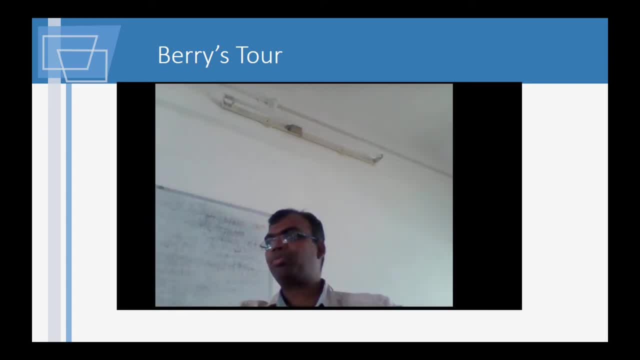 And it will be columns. The roof might be a dome or it might even be a flat roof, And it's. you have to think of the buoyancy of that. You have to think of the buoyancy also. That is when the tank is empty. it should not float up. 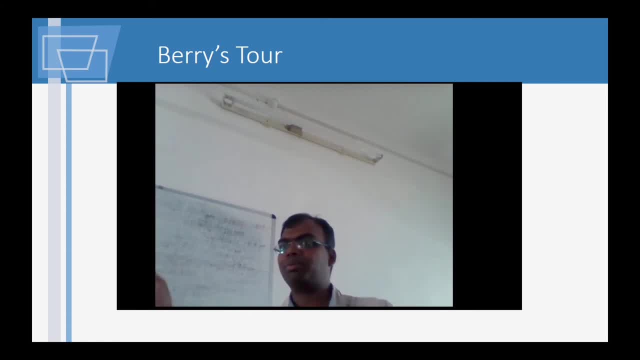 And the float tanks cannot be cast in one piece. So there are watertight joints which have to be thought of And there's a base wrap column and this one connectivity crack with this important criteria. So, in case you are going to relate it to your structural design, these are some of the factors which you'll have to take into account. 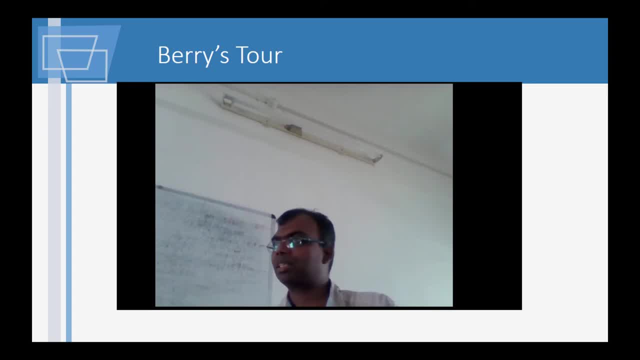 So all these columns and everything will be coated with some material for watertight joints, Some material for watertightness which is also non-toxic, So this: such tanks will be there near each water treatment facility. Then it is taken to the overhead reservoirs, from where it is pumped. 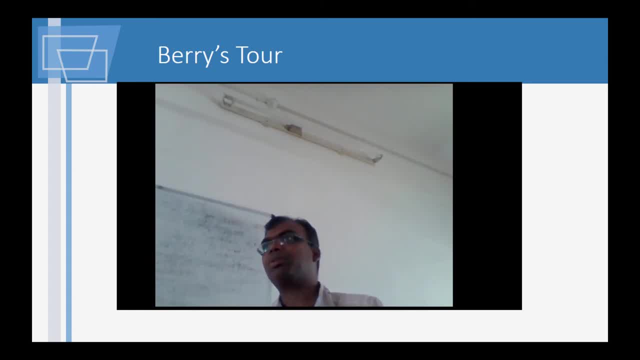 Usually you'll only see the overhead reservoirs, But there's also very big underground reservoir near each of these overhead tanks. Okay, So I'll just like to also just have a look at that. Okay So let's look at our syllabus. 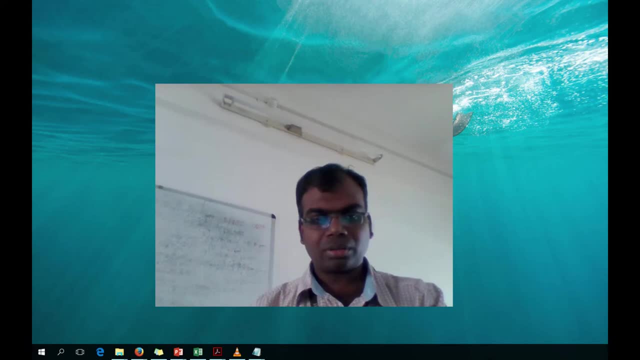 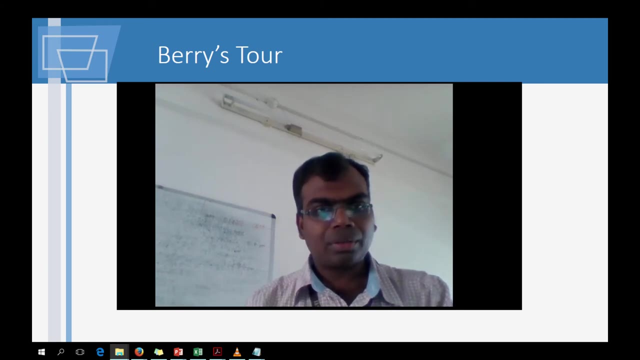 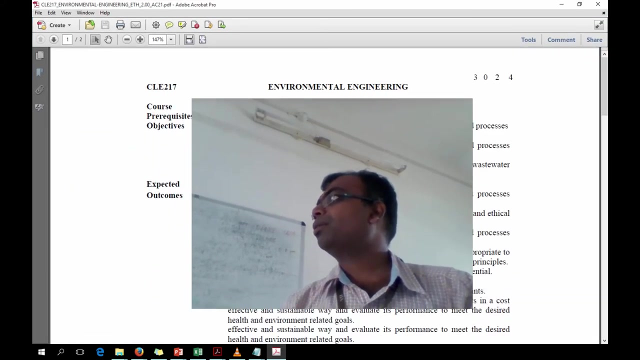 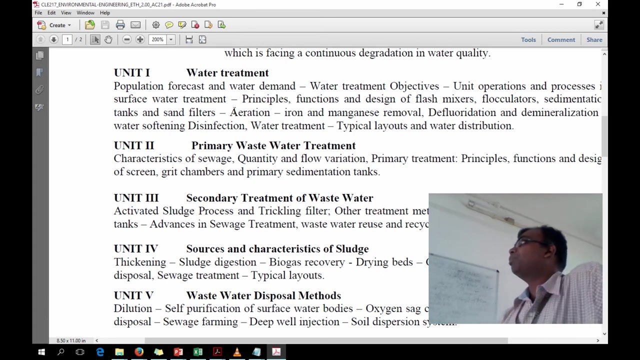 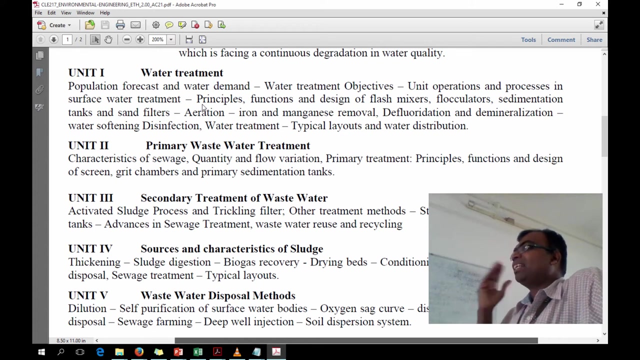 So let me open the syllabus, Yes, Okay, Now of the syllabus, we saw the population forecast and water demand. We had a look at the water treatment objectives. We also saw the unit operations and processing. Now, if they look at the water supply, water supply and the water supply май be compared to the water supply model. 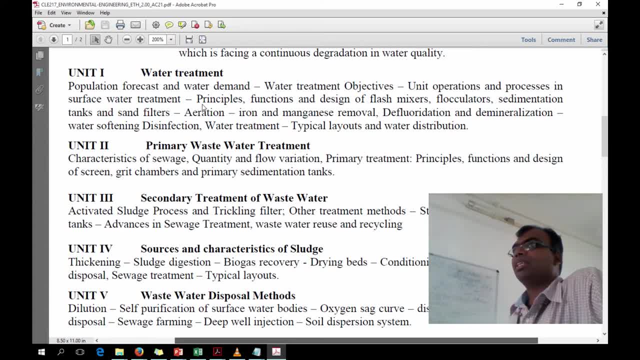 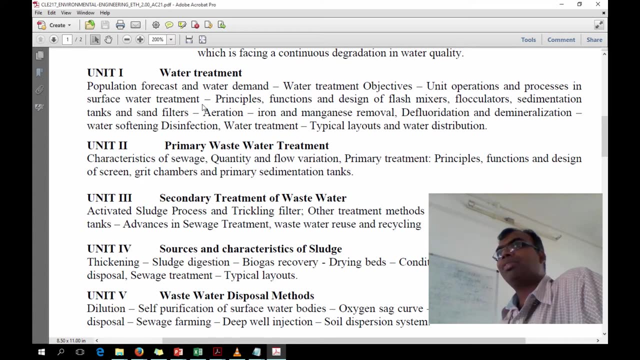 You see the water supply. the water supply is very different from the surface water treatment Of the. You know the water supply is different. The water supply is different from the surface water treatment. important if you are, if you are drawing the water from a place which is very 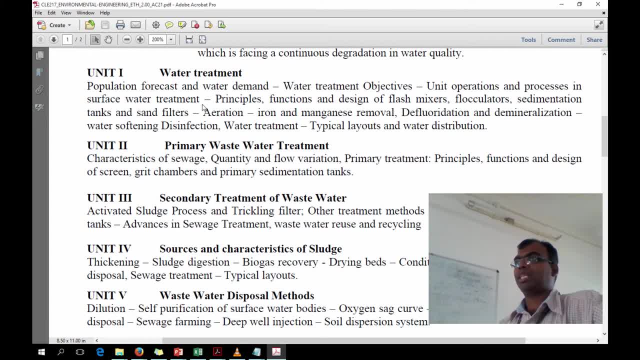 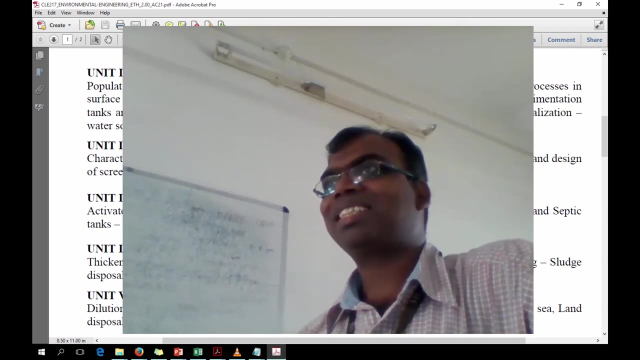 very warm, the chances are that a lot of biological growth could be there. so temperature also controls the amount of dissolved oxygen. what happens when you elevate the temperature? devo will increase or decrease. increase, okay, how many of you have had boiled water in your childhood days? at least did you. 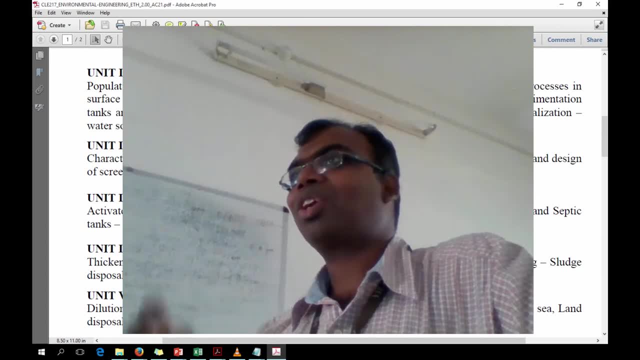 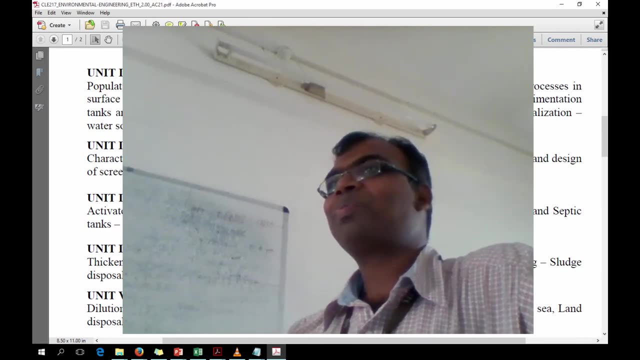 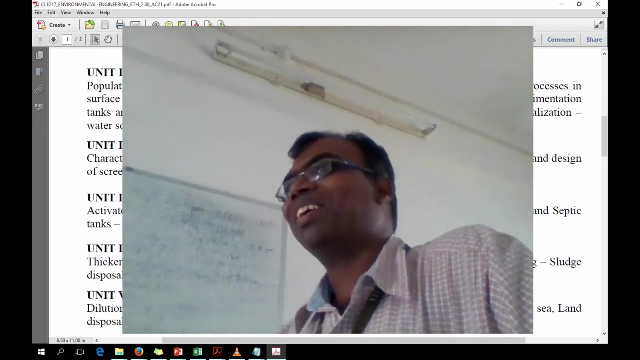 like the taste of boiled water or raw water. raw water, why was raw water taste here? okay, yeah, that reason is dissolved oxygen. if you boil it, the oxygen is pushed out. when you are at elevated temperature, dissolved oxygen reduces impact. okay, so I just wanted to point it out to you. when you elevate temperature, dissolved. 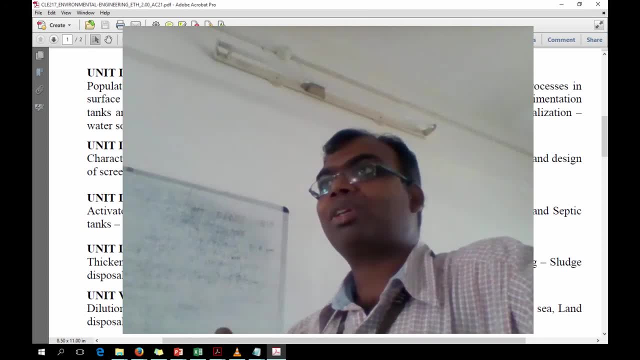 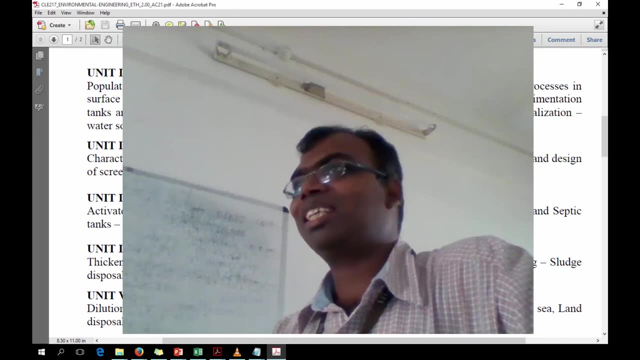 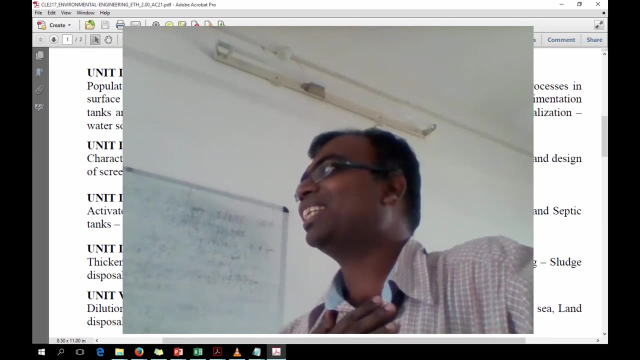 oxygen comes down. so, in fact, when you have water, hot water, bath in your this one and you are sending it into your drain, one of the things you are also doing is, already the dissolved oxygen is less in your drain, you are making it even lesser. it becomes more septic. of course, I also bathe in hot water. I shouldn't be telling much, but I do feel guilty about it. but this is the fact that happens, and the only way you can bring it back is by agitating the water or something where you introduce the atmospheric air into the water again. so this is the reason why you are boiled: water doesn't taste. 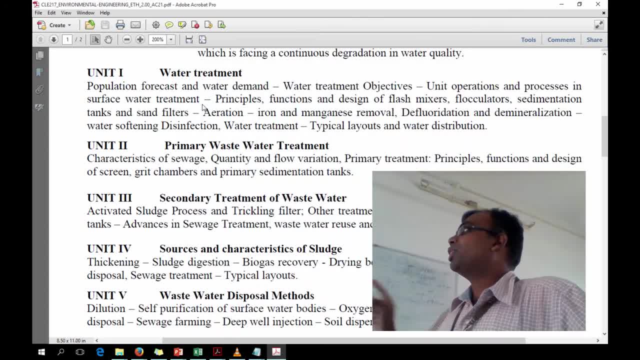 all that good here. so then we have the principles and functions and design of flash mixer. so the principle of flash mixing is: it is done rapidly, is done rapidly so that the chemicals are mixed, flow okay, so function. also it comes for the flash mixer. and then you got flocculators. they are 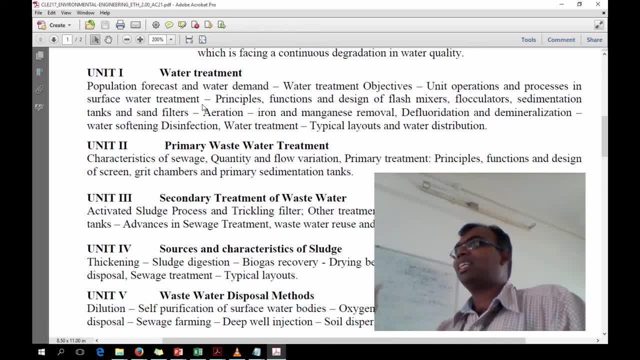 to be at a particular speed. solar flocks form. Too less energy is not there for flocks formation, too much it will break it into pieces. ok, Sedimentation tanks, it can be just gravity settling which is there, or you can go for the thickness sort of clarifiers which have. 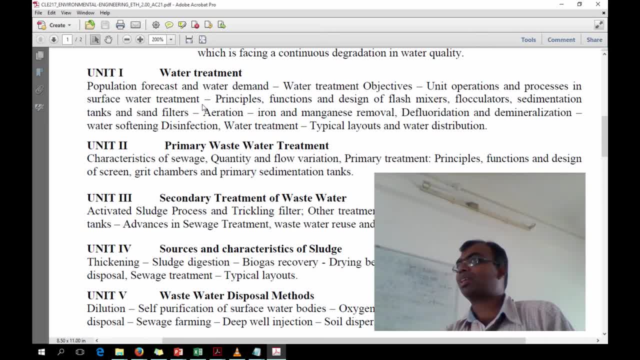 a different, built itself The aerator. remove what Flocks? yes, ok, but I am talking about sedimenting large pieces. sedimenting large pieces, ok, Aeration, two things. one: you increase the dissolved oxygen levels. it might be it will be also in disinfection process and also. 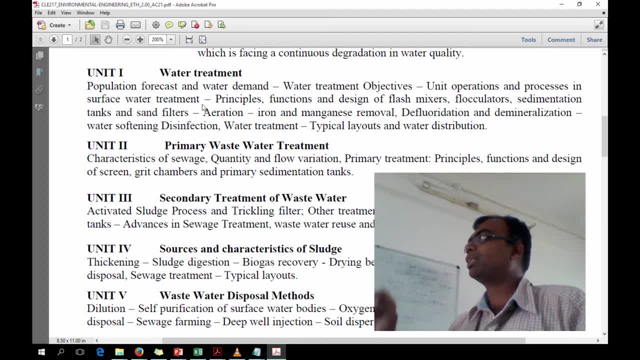 it might be a requirement for a process. Please remember, aeration can be also a process requirement. So, for instance, if you are going to go for biological reactors, which is aerobic, you need to have dissolved oxygen in the system. Iron and manganese removal. I have not this chemical. 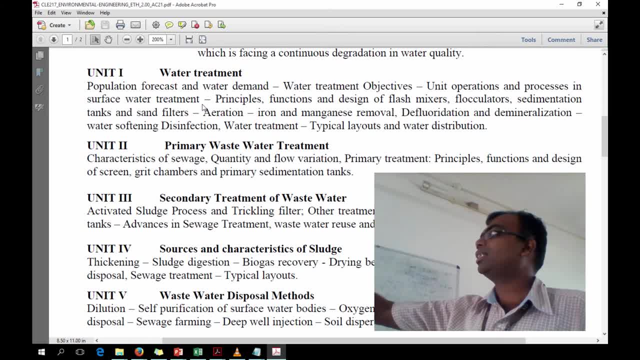 reaction. So things I have not touched, ok, Next lecture I will definitely do it. iron and manganese, depluritization, demodulation and water treatment: ok. And second thing is very, very simple: this unit operations. with your permission, I will not be dealing too much. ok, in the second unit. 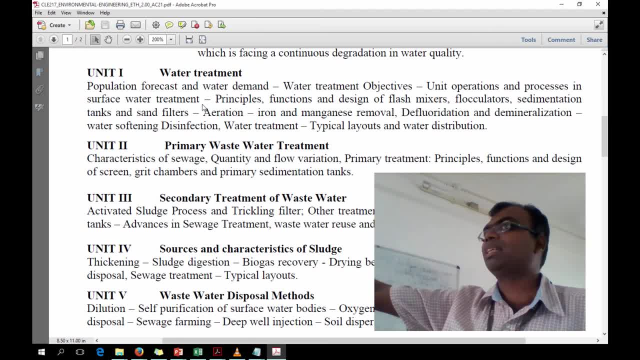 Principles, function and design of screen. bar screens- ok, Grid chambers. bar screen and grid chambers are very similar. Bar screens are the are just bars which will not let wood go through. The grid chamber is something like what we saw in this one, like he was talking about fish. you know not getting caught right that. 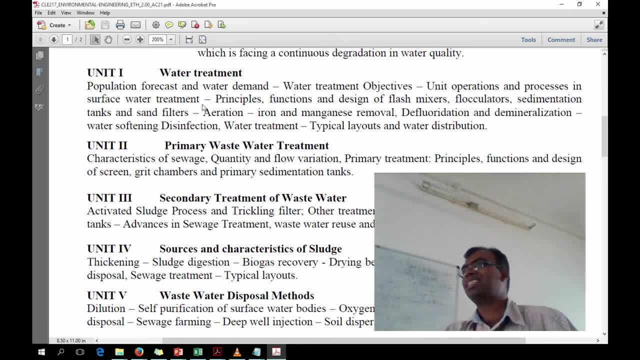 sort of thing is a grid chamber And primary sedimentation tanks. they are just large tanks where the velocity of water is brought to such a level that sedimentation will take place. Please remember: whenever there is a lot of energy, the material cannot sediment. that is a very fundamental principle. Water still will not get sediment. that is a fundamental 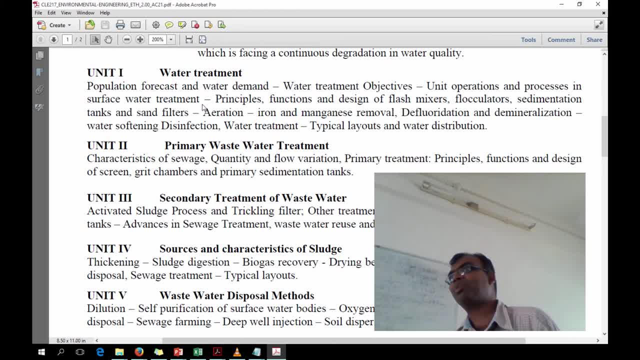 principle. Okay, Thank you very much, Thank you very much, Thank you, Thank you, Thank you still looks clear. By the moment a child runs into the water, it starts to get turbid. ok, So if it is clay, it will become very turbid. If it is sand, you can see sand mixing. but 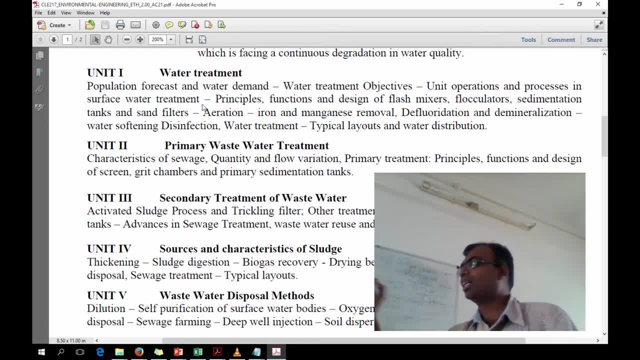 it will again settle as soon as energy is not there. So the larger the particles, settling is faster. That is why we go for all this flocculation and other techniques. ok, So basically I was thinking that 3 units was doable. However, I am going to still stick. 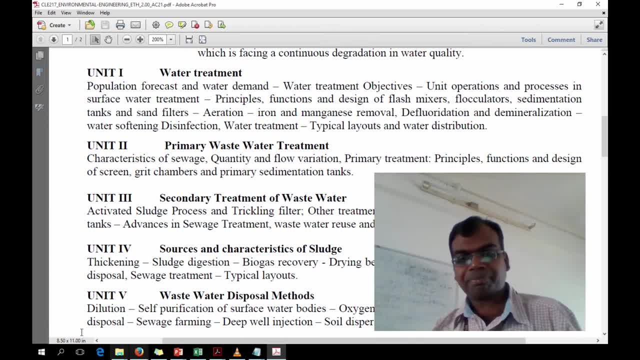 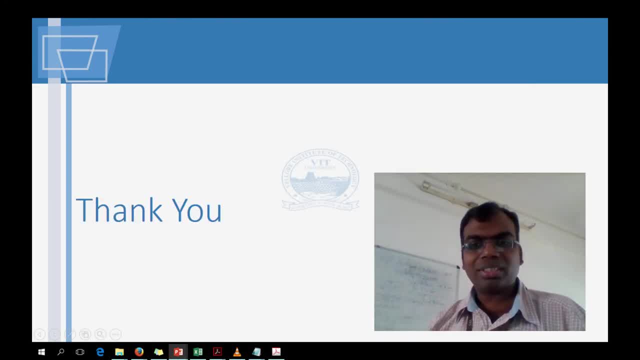 to 2 units for the exam. ok, Now I will stop this lecture saying thank you, ok, And we will just discuss what we are going to do for our assignment for today, ok.